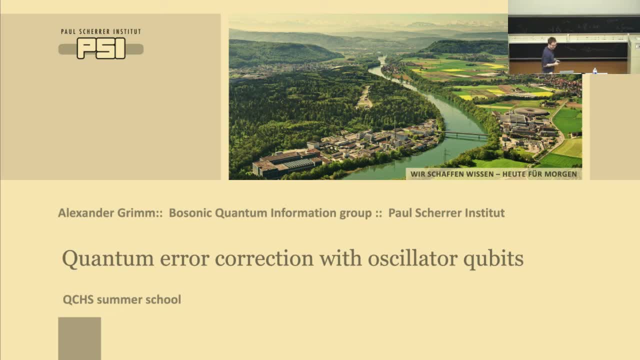 Yeah. so this fun fact, of course, is only a fun fact. many years after. I'm glad that it worked out and now I am starting my own research activity at the Palscher Institute. As was said, we are the Bosonic Quantum Information Group. 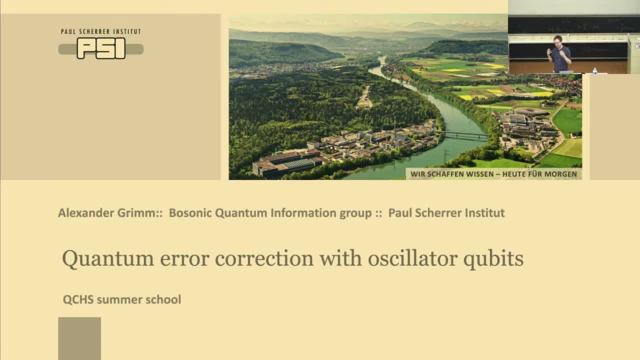 We are part of the PSI quantum effort. We're not part of this quantum hub. There's a separate superconducting circuits group in that, just in case there's any confusion. So what I'll speak about today are these oscillator or Bosonic qubits, right? 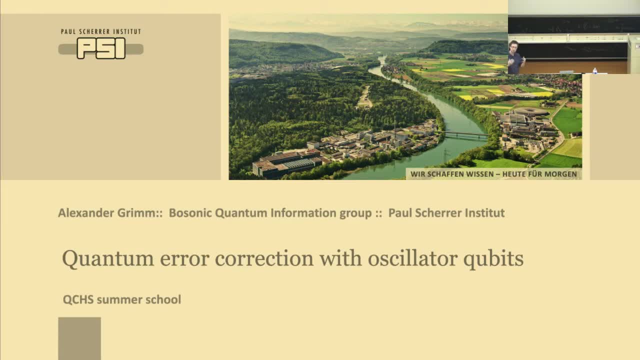 And they are a way of hopefully reducing the hardware overhead that's associated with quantum error correction. Cornelius has already introduced this nicely earlier and I'll give you two other examples. He's talked about this GKB code. I will give you two different code examples. speak a little bit about how the encodings work. 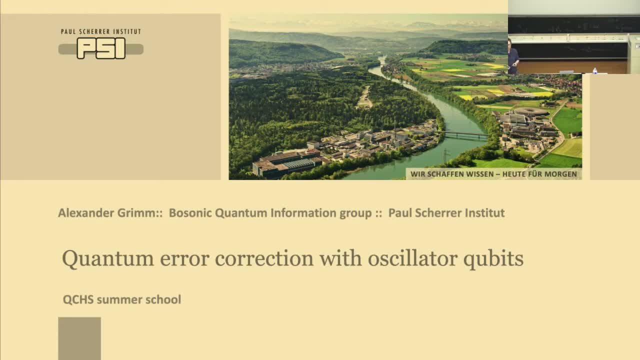 what the error correction capabilities of these are and how they're implemented, And what challenges do we still have to face? So there's been a lot of nice explanations that you've had on quantum error correction and superconducting circuits yesterday and this morning. right, 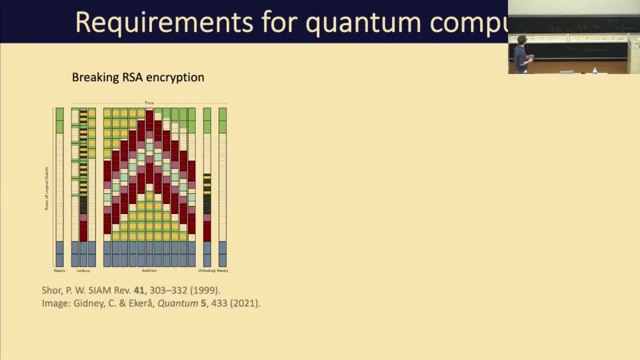 So I will be able to build on this work. Nevertheless, I also want to say a few words just about different requirements for quantum computing or typical applications that people have in mind. Bear with me on that. I'm using this to make a point. 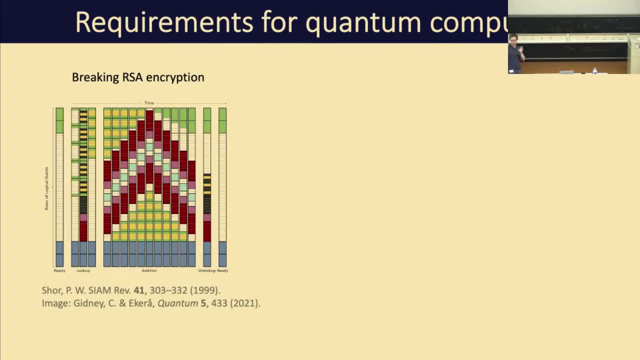 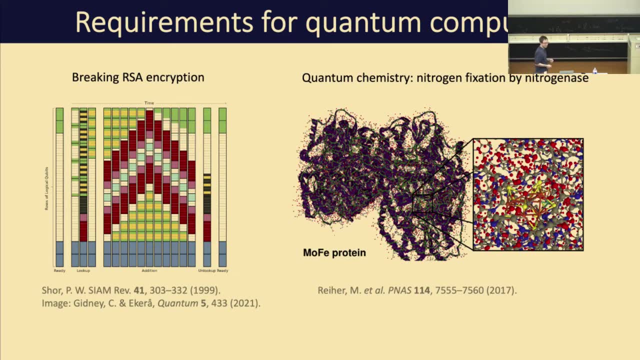 So, if you think of different quantum computing applications, where you really think of applications of a universal quantum computer, right, There's this RSA encryption breaking, and then there are other, maybe a little bit nicer applications, such as this quantum chemistry simulation, where this paper was published in 2017 by the group. 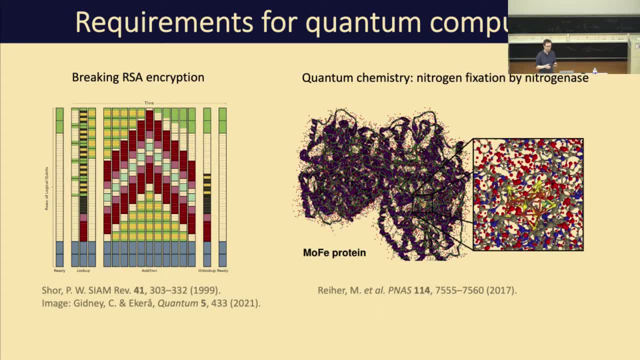 of when he was at ETH, where they found a way how a universal quantum computer could help us to understand chemical processes that happen in soil bacteria when they pull nitrogen out of the air to make fertilizer, And they can do that at ambient pressure. They can do that at ambient pressure. 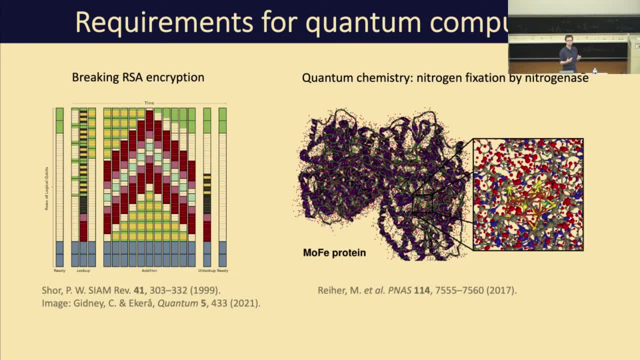 They can do that at ambient pressure, Ambient temperature. We can do that If we understood that. it would, of course, be really nice, But it's also good to always perform a reality check on these things. right, And so for these two applications, you need somewhere in between 100 and 10,000 logical qubits. 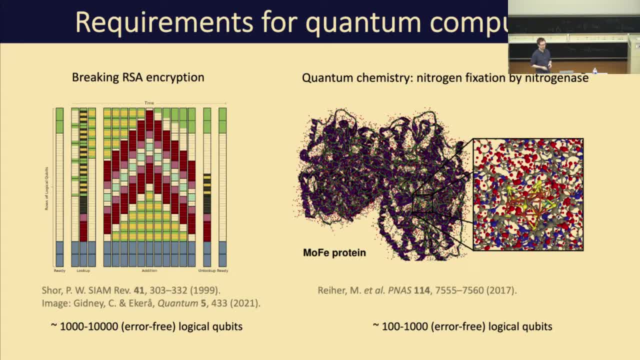 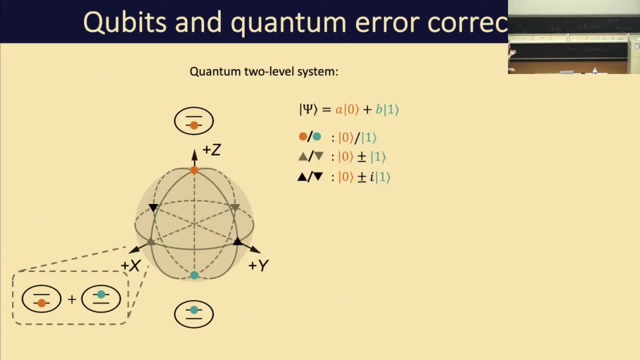 And these are supposed error-free right And our current qubits are from error-free. We've heard this time and again. If you think about a typical way of implementing a qubit right, You would do that with a quantum two-level system. 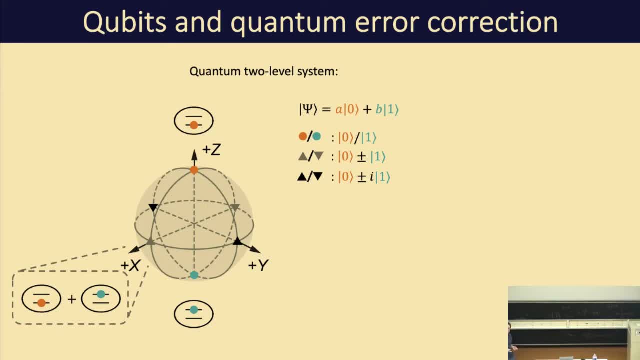 where you encode the information into superpositions of the ground and excited states And such quantum two-level systems are to some extent, you know, intrinsically fragile because you want to couple to them right. We've heard that too. 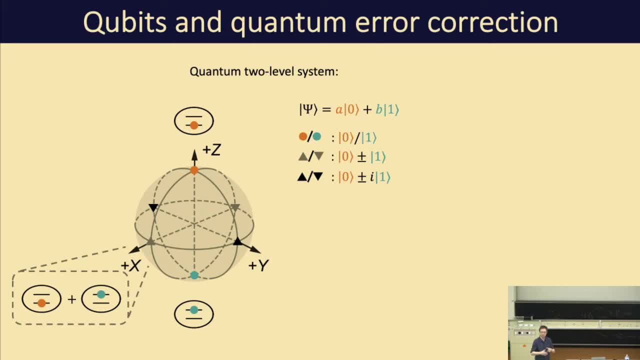 And if you couple to them, if you put our grubby classical hands on these qubits, then other degrees of freedom can also couple to them And you might lose this quantum of excitation or you might gain one if your environment is at a finite temperature. 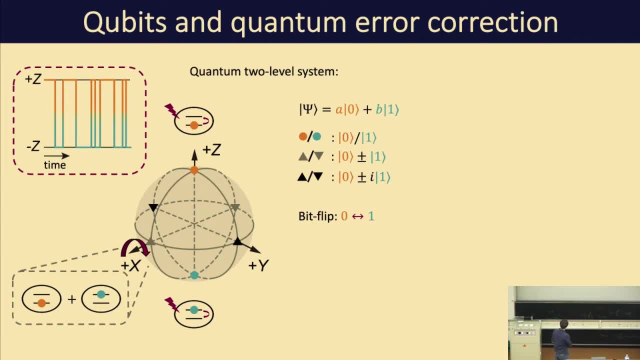 And what then happens is that you flip along the z-axis Or equivalently around the x-axis of this qubit. I'm simplifying a bit here, But in the context of what comes next- quantum error correction- you can think essentially of one type of error that happens on such a qubit. 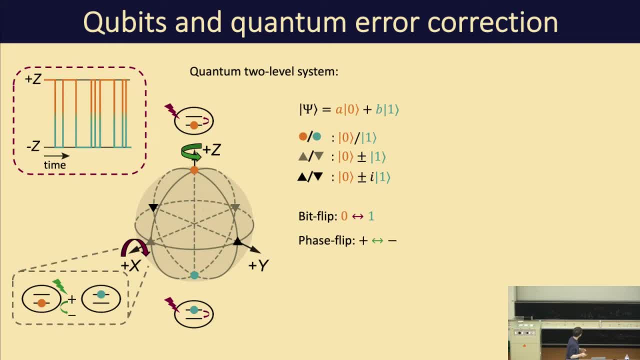 as a bit flip that flips the zero and one value, And then of course, you also have phase flips. You've heard about those where you flip the sign of the superposition, And you've also heard about how we can tackle this with quantum error correction. 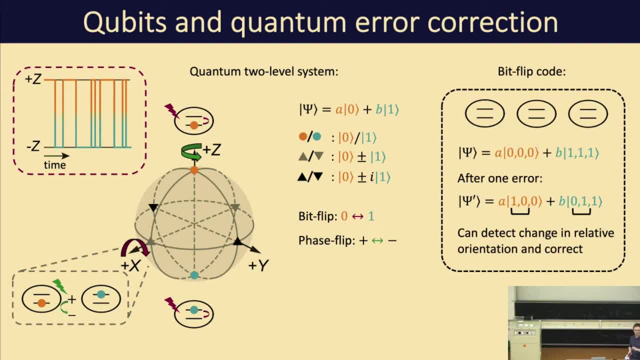 This example I think you've seen for the third time now, so I can go rather fast on this. That's the bit flip code. It's a bit flip code. It's in some sense the simplest explanation of how such a code could work. 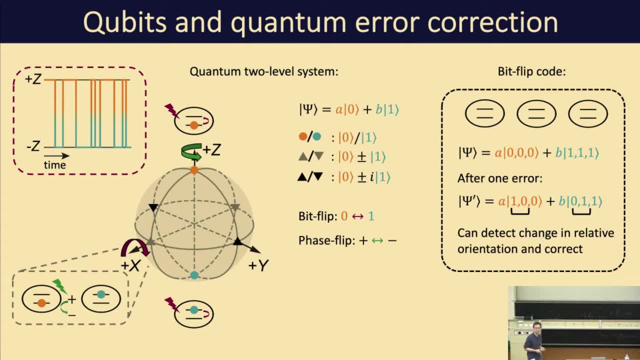 where you introduce redundancy by using a state of physical qubits now And you measure these joint quantities, these periodes- Christopher called them this morning- that allow you to detect errors without actually projecting into any of these two states. So your quantum information is still safe. 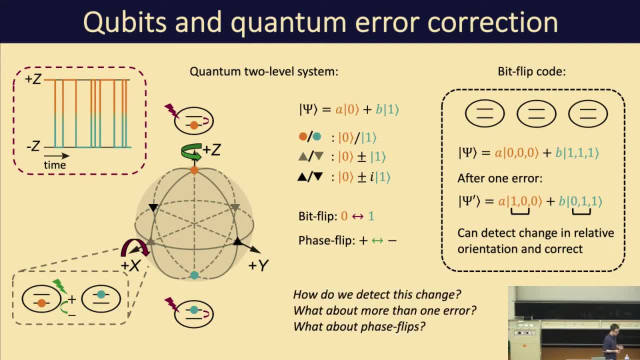 And that's a nice example, But in some sense it always raises more questions than it answers. Some of these were already answered this morning, So again, I can build on what the previous speakers have said. Now, how do we detect these changes right? 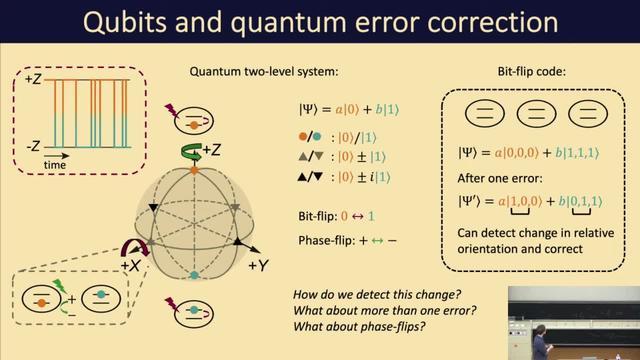 We have to use auxiliary qubits that couple to these data qubits. And if we want to correct for more than one bit flip again, we have to make the chain larger. If you want to correct for phase flips again, you have to introduce more redundancy. 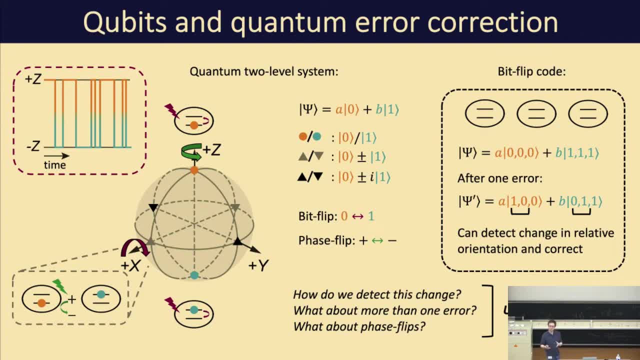 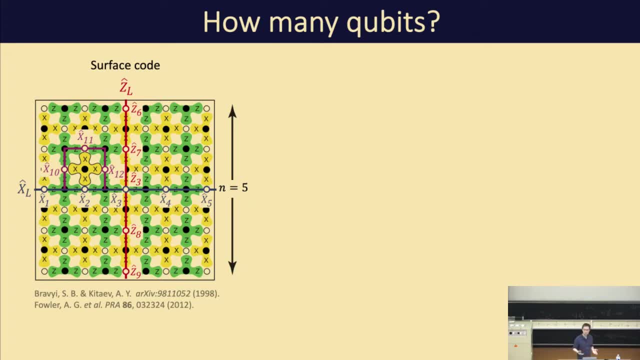 So in this paradigm, the answer is use more qubits, right, And that is not a bad answer. That's, in fact, an excellent answer. There are really good codes and ideas for this, the surface code. you've heard about this. 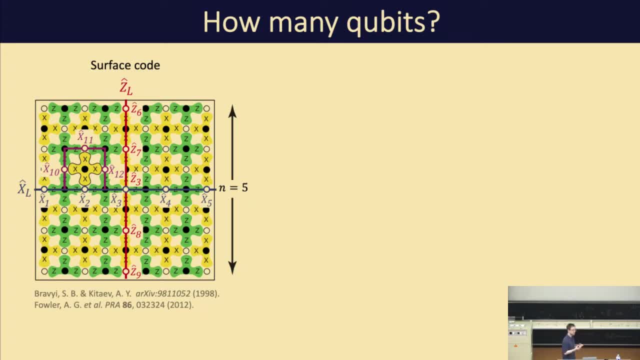 Also where you now can correct for bit and phase flips in a paradigm that's fault tolerant and so on. And in this example here, for instance, you have these data qubits, which are the open circles, and the measurement auxiliary qubits. 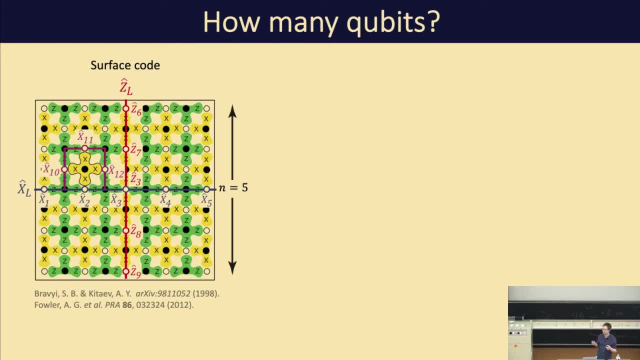 that are these black dots that measure these four-way correlators. And your logical qubit now, in the simple example, would live as an entangled state of this entire grid, where flipping the logical qubit around the Z-axis requires flipping all these five qubits. 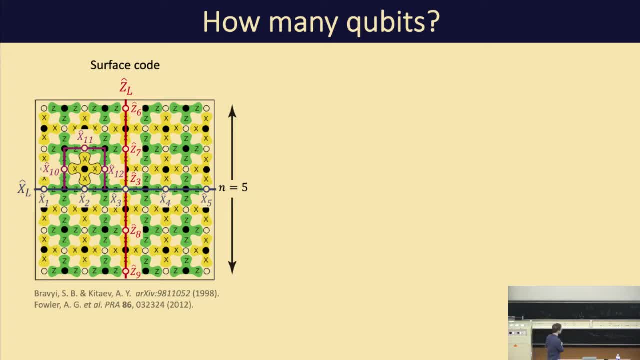 And that is the way we use it: data qubits: flipping it around the x-axis requires flipping all these five data qubits and that's easy for us to do, and our assumption that hopefully is true is that it's hard for errors to do, because errors tend to act locally and 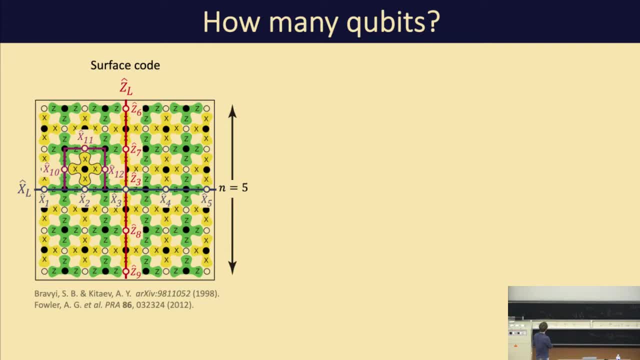 not globally right. and so if you make this distance, this number of qubits that spans one side of this, this square, larger, then your error prediction gets better and better. so that's one way to think about this, and that now also supplies us with a way to think about how do we get from our current physical 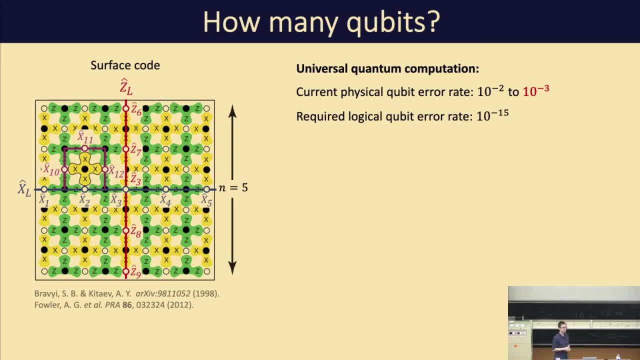 qubit error rates, which are, at best, I would say, 10 to the minus 3, especially if you think of two qubit gates here. this error rate is the probability of suffering an error during any given operation, right to the ones that we would need for the examples that I've given you earlier, where you really see 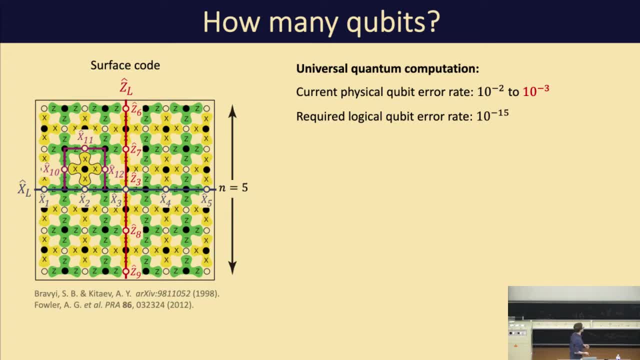 there's quite a few orders of magnitudes to go. so making this grid bigger, how big? well, for this first example I've given, you need about 20 million physical qubits at these various state-of-the-art error rates. for the other one, you need 180. 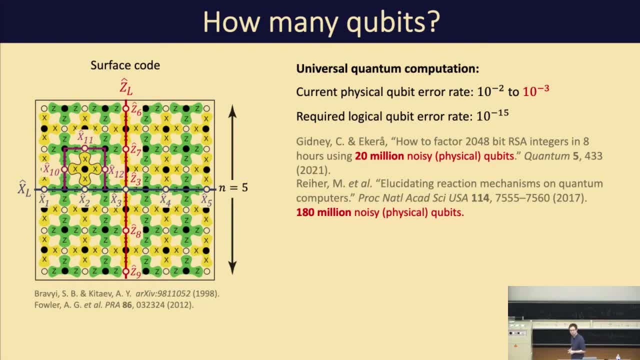 million. so that's a lot, that's really a lot of qubits right, and I think that really nicely shows that this is a marathon not a sprint. Cornelius has nicely said that also earlier, and I'm not saying we can't do really nice things in the meantime while we get there this noisy intermediate scale. 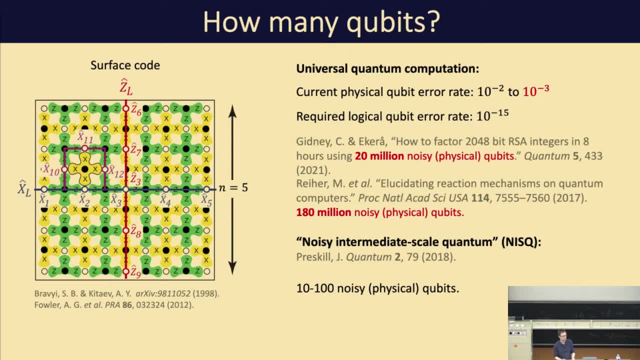 quantum paradigm allow us to do nice experiments with tens or hundreds of physical, noisy qubits. there may be more experiments than we, as in my opinion, that we as physicists care about. you know Adobe simulations and so on, but these applications that are also cited as applications for quantum computers, where we are very confident that there's a 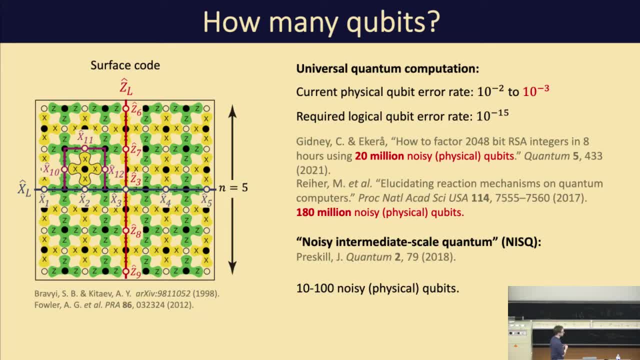 speed-up for useful problem. they do have a really high overhead, and so it's absolutely justified, I think, to think very hard about how can we reduce our this overhead. this can be done on the theory side. you can come up with better decoders for your error syndromes and so on, so these numbers do get lower just by. 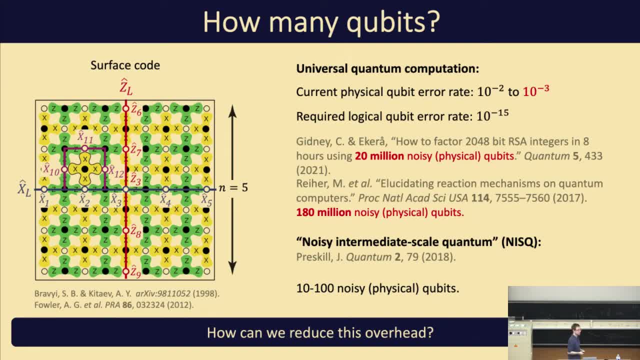 theoretically, finding better ways of doing your quantum error correction, but it can also be done on the hardware side by making your physical systems better. and the route that we're taking- and I think that you know is quite interesting- I would like to tell you about today is that we'd like to rethink what the 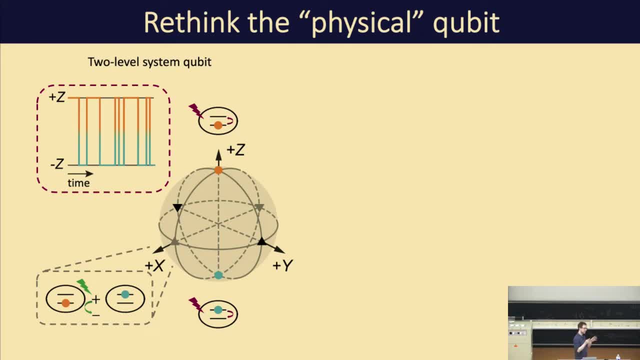 physical qubit should look like. this is now, of course, with a superconducting circuits focus right. I told you about the two-level system approach earlier. now we can contrast that with how a classical bit works right. a classical bit is pretty stable. it involves many quanta. it's encoded in what you could. 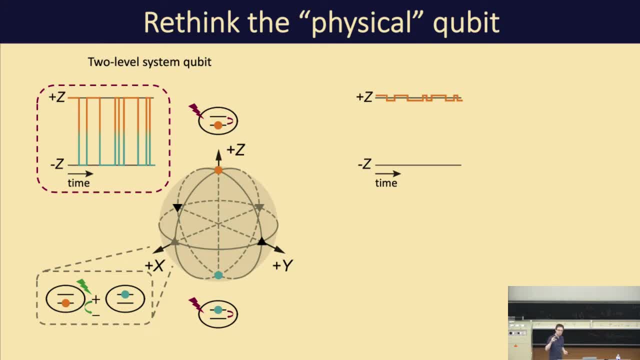 call microscopically distinct states. if your environment comes and it messes with this qubit, exchange a few quanta, right, it's not gonna really care, it won't flip from one value to the other, and you can extend that to the other, and you can extend that to the other, and you can. 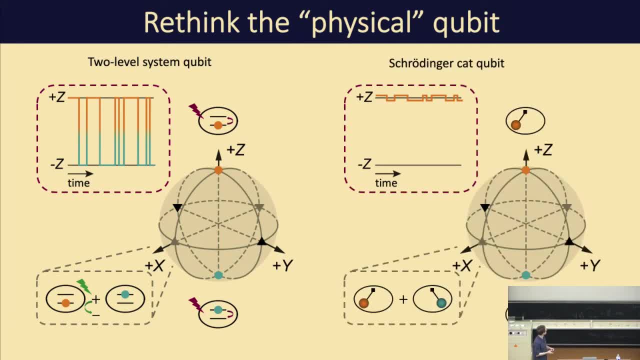 this paradigm by saying: now you're encoding a qubit into superpositions of macroscopically distinct states. such a qubit is called a Schrodinger cat qubit. there's an analogy with, you know, this thought experiment with the poor cat that's in the superposition of the macroscopically distinct states of being. 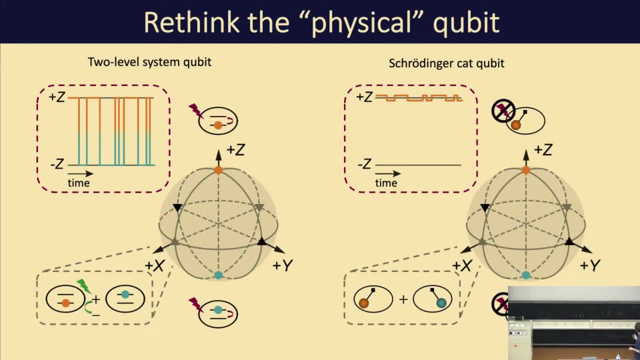 dead and alive. so now, what you'll gain from that is you get one axis of this qubit that is protected, because here you have this macroscopic distinct states, and then the other axis you have to deal with later, at least for this first example that I'll talk about. right, so the first example that I'll talk about is: 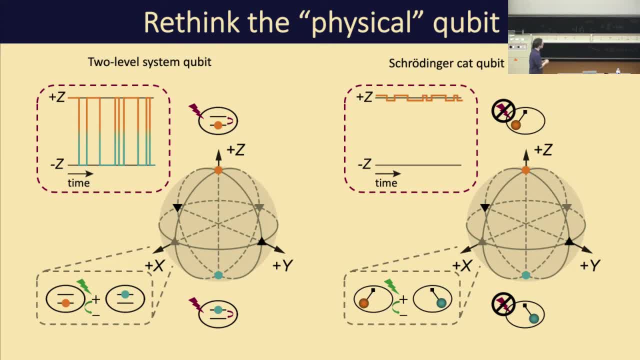 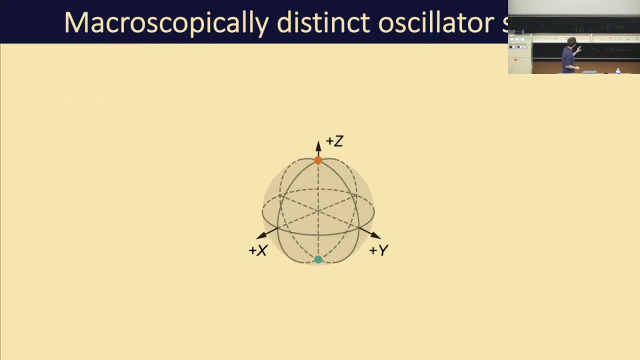 the hyperposition, and the hyperposition is actually the only thing that you can talk about, right, because you're not doing anything about the fragility of the superpositions. in fact, you make it a little bit worse now. first I'll comment on that also in more detail. first let's speak about what are good candidate. 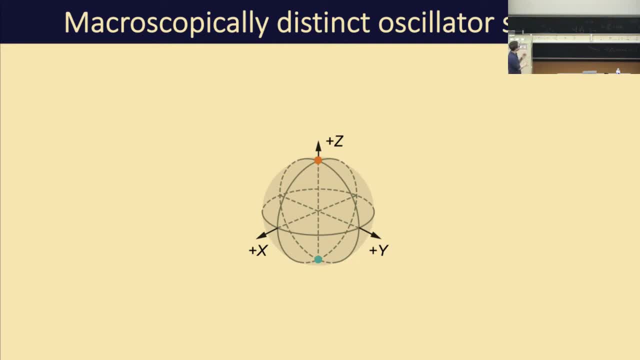 states for such macroscopically distinct states. good candidate states are microscopically distinct, oscillator states why? well, you can think about such states as oscillations of a pendulum. let's consider these two oscillations: one where it started, on the right, so they just have different phases. Now this: 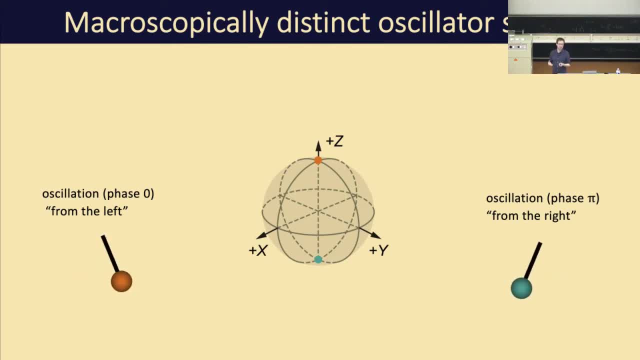 might seem pretty similar to you, but they're really quite distinct. Think about what you have to do to switch from one to the other. You have to really grab the pendulum, hold it for half an oscillation period and then kick it off again, and that only switches between these two, And that is a big perturbation. 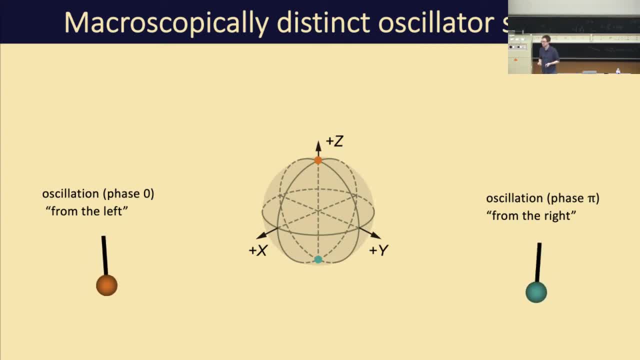 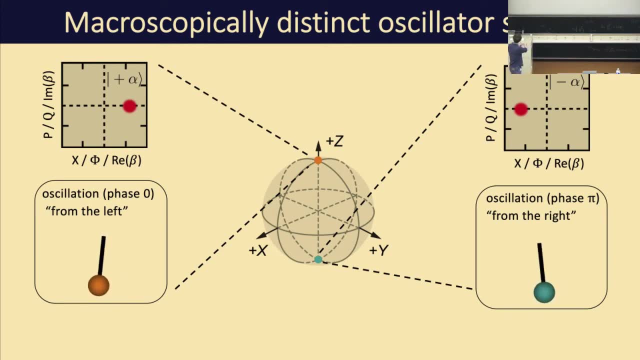 to the system, and that's also true for typical noise processes in an oscillator, Best illustrated by looking at the phase space of the oscillator. So let me just remind you a bit of this phase space. Here you have the one quadrature which could be position, the other one could be momentum or, in our case, we 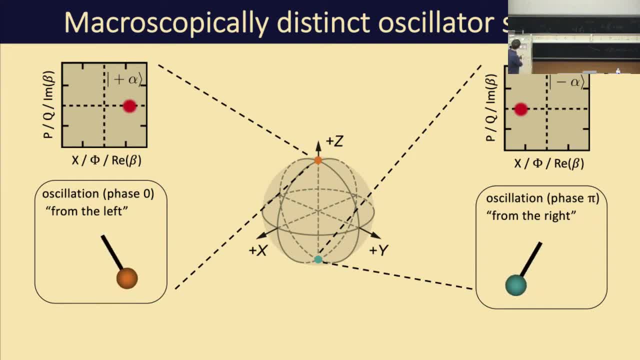 experimentally work with superconducting circuits. So the quadratures are going to be an effective flux through an inductor and the charge on a capacitor, or we can just say real and imaginary phase space coordinates. Such an oscillation in our language corresponds to a coherent state that has a fixed position in this phase. 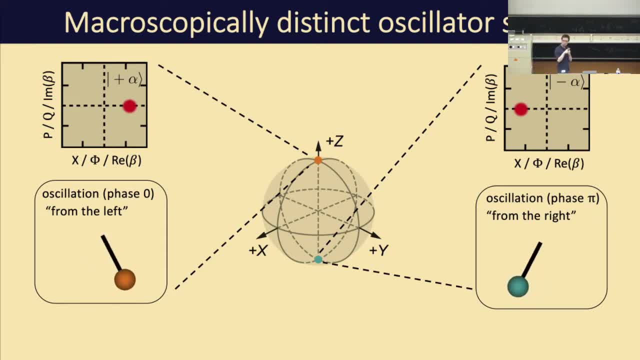 space. It's a disk, not a point, because of the Heisenberg uncertainty between oscillations. The two quadratures that you get and its distance from the real axis gives you the amplitude of the oscillation. its angle with the real axis gives you the. 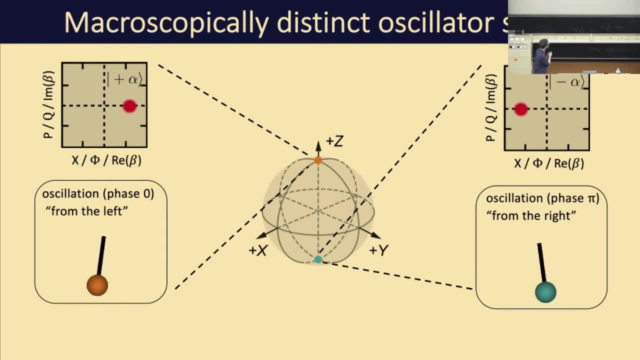 phase of this oscillation. So here it's zero and here it's pi. Now these two states are distant in phase space and that's where this error protection or protection against typical noise process is going to come from. If you think about typical noise processes in an oscillator, you have D-phasing, where you just 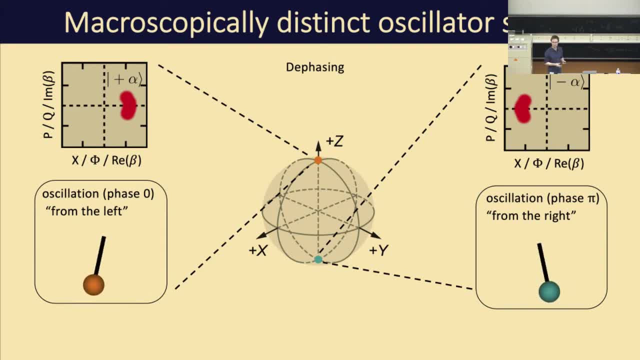 randomly wiggle around the oscillator and then you have the phase space, which is the phase space, And then you have the phase around the frequency of the oscillator and that randomizes the phase along a circle around the origin right, and so this gets smeared out. You see that on short timescales these states can stay. 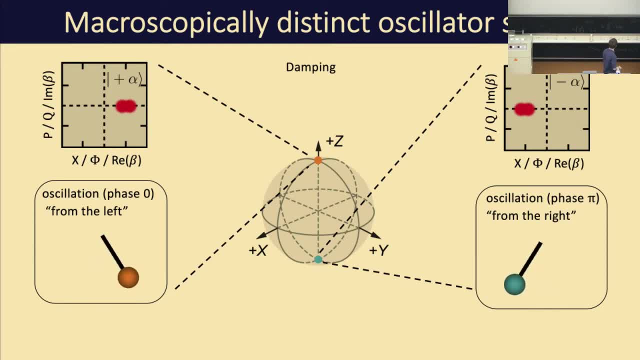 distinct. Now, another noise process that you can get is damping, where the states decay to the origin. that's it actually has two parts of damping, if you think about it quantum mechanically. there is a deterministic decay to the origin and then there are random photon jumps. I'll talk about the random photon jumps. 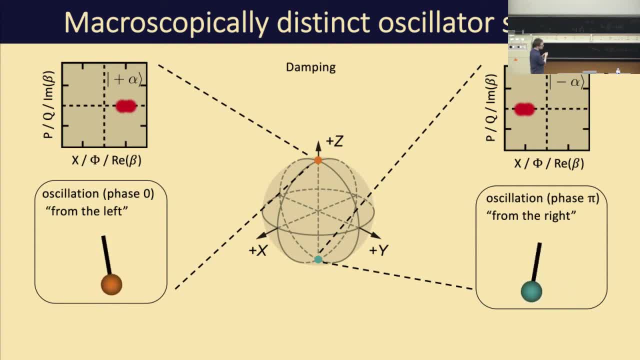 later Here I'll talk about this part first. So this deterministic decay, also in short timescales, is not going to make your coherent states overlap. So there's the potential to correct for these two different noise processes and there's a potential here to essentially implement. 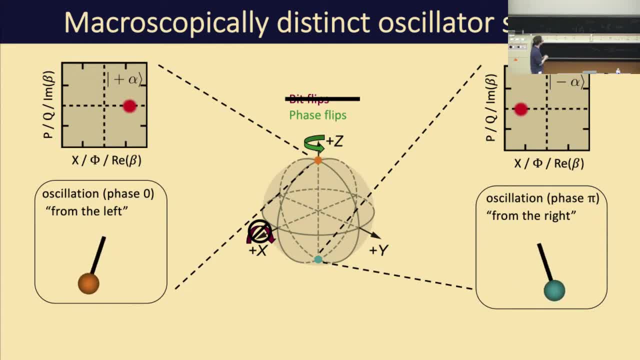 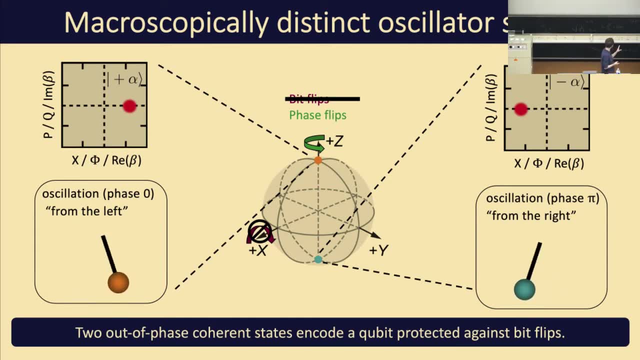 the qubit that doesn't have bit flips, or where bit flips are strongly suppressed and only phase flips are left. Now that's my take home from this slide. You can encode a qubit that is protected against bit flips into these two coherence states, which are distant in phase space. 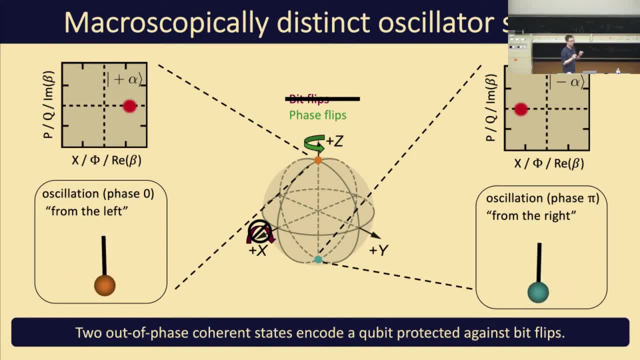 But that's only half of the story, really, because I talked about the short timescales regularly and what we really need is long timescales. of course, right, We want to find some way of pinning these states in place of stabilizing them, and that's where all the magic happens, in some sense. That's where I 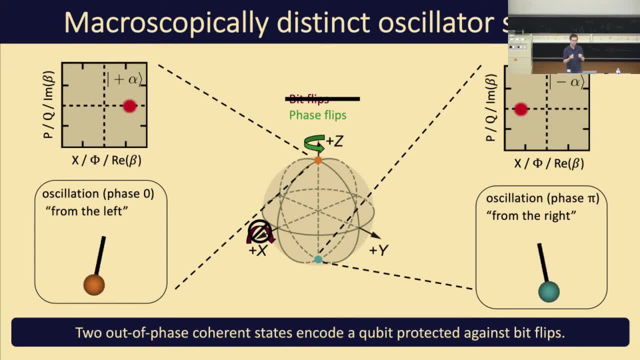 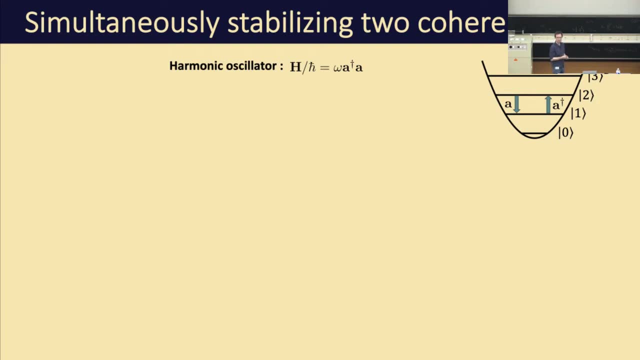 have to come up with smart circuits, smart processes that engineer a kind of dynamics such that these two coherent states are simultaneously stable, all of their superpositions. Now, how do we do that? Well, we start. we could start with a harmonic oscillator, but a harmonic oscillator by itself can. 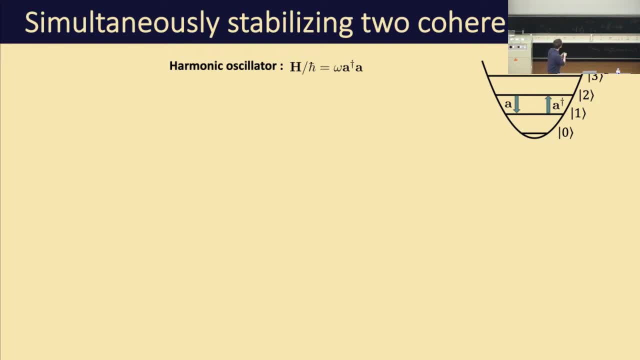 really not create, you know, non-classical, non-Gaussian states. So we have our harmonic oscillator with this harmonic potential, the photon Fock states in here and the ladder operators that go up or down. Here's the Hamiltonian with the corresponding frequency. Now, if you apply a coherent drive to such a system, that's. 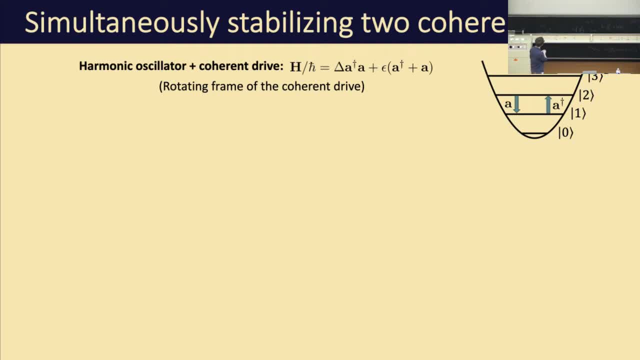 the coherent drive. and here we've gone into the reference frame of the drive where it's applied with the detuning. So this first part here is now showing the detuning of the drive. What you will get is a superposition of these photon Fock states. that corresponds to a coherent state, but just one, and it has a. 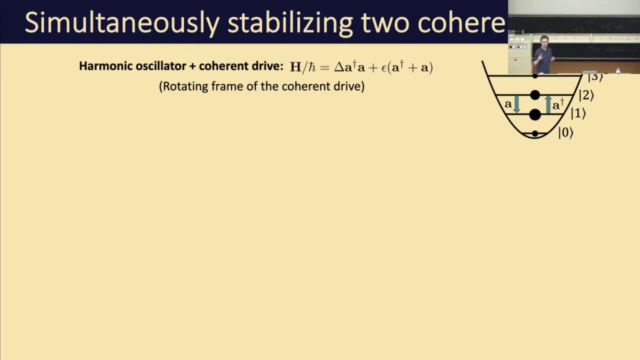 well-defined phase and amplitude. What we want is two, and so the trick that we're playing essentially is we square all these operators here and now we get a photon number dependent detuning and we get a single mode squeezing drive, which is like a coherent drive, but it exchanges two photons with the system. 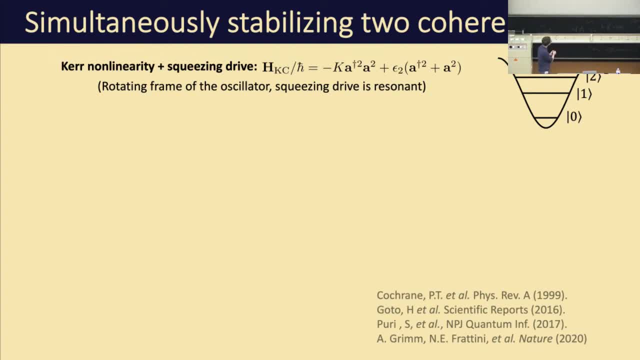 at a time instead of one. Now, this is, as you might notice, essentially an anemonic oscillator that's being driven. You've seen this on an earlier slide, on Christopher's slide, The bottom two levels of this are also implementing transmon qubits in superconducting. 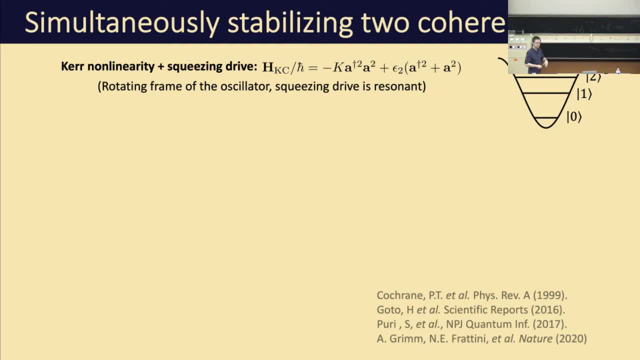 circuits. What we're doing here is we're adding this additional drive and this now gives us access to a dynamic that creates essentially a quasi-potential in phase space. that looks like this: Think of this like a classical way of plotting this: Hamiltonian. here You have two extrema, and these two extrema correspond. 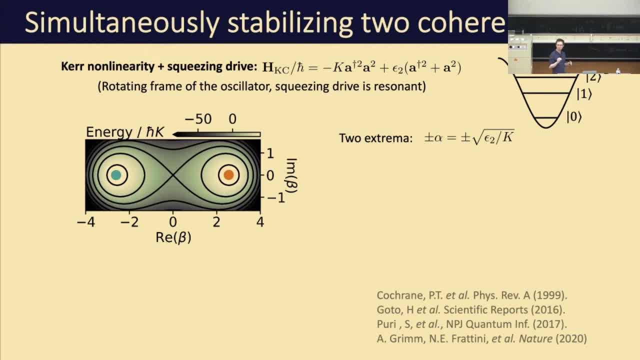 to stable, steady states. sorry of this dynamics. Now that's classical. They sit at these two amplitude plus minus, square root of epsilon 2 over k, but also quantum mechanically this remains true. If you take this Hamiltonian and you factorize it in this way, you can see that this second parenthesis here is going to. 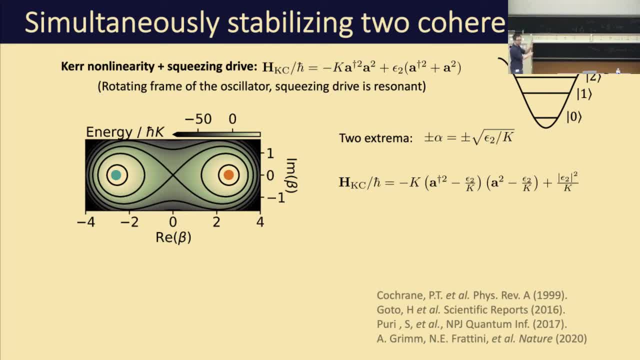 annihilate these two coherent states, plus and minus alpha, with these given amplitudes here, and that's based on the fact that these coherent states are eigenstates of the annihilation operator. So a square is going to bring out a value, alpha square which corresponds to: 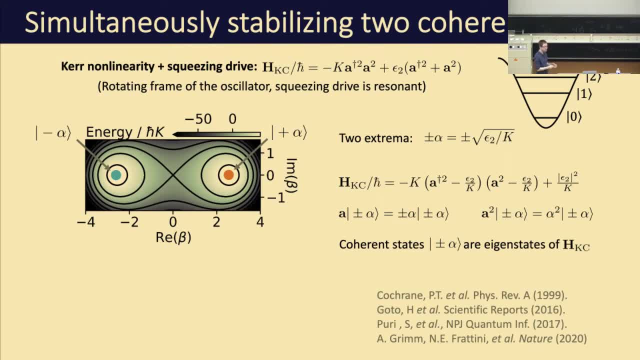 epsilon 2 over k. Let me say in passing that all of this is really based on the fact that we use this a squared operator. if we just use this normal a operator like the equation I've shown you earlier, it would be able to distinguish between: 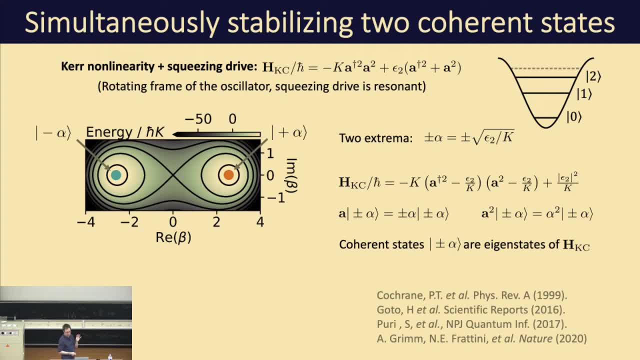 these. So these two coherent states have fixed energy with respect to this Hamiltonian. They are eigenstates of its evolution and they are stable, and that's also true for all their superpositions. It's also the case that there's an energy gap that separates all the other eigenstates from 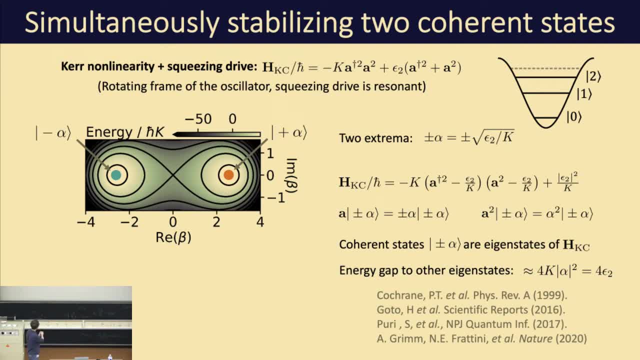 these coherent states and their superpositions. That's very hard to move from one to the other. in a nutshell, Now, that does all the things that I should say that this way of stabilizing it, which is called the Kirchert approach, has been implemented by us, but there's also other approaches where you engineer. 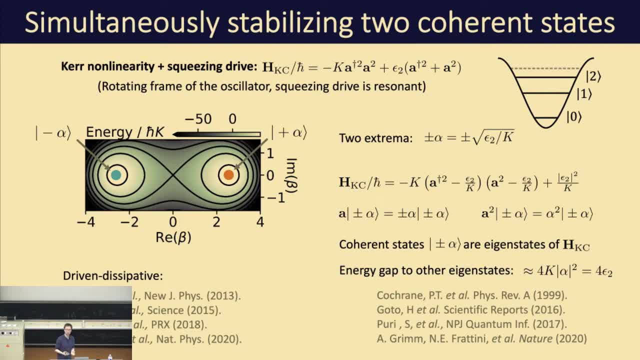 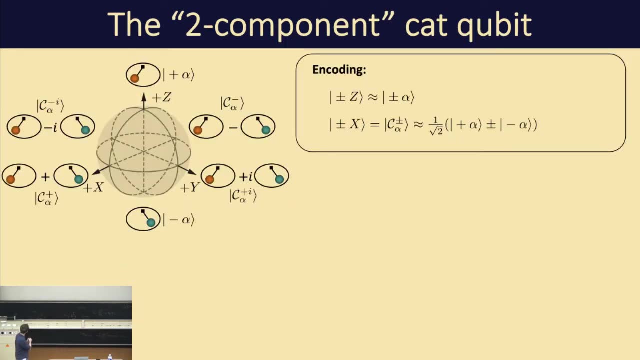 nonlinear drives and dissipation that have a similar effect, and there's a lot of interesting work coming out of that. It's a very active field with very lots of new results. But that being said, maybe let me talk a bit about the encoding that we're using. How does it look like? Well, I told you along the Z. 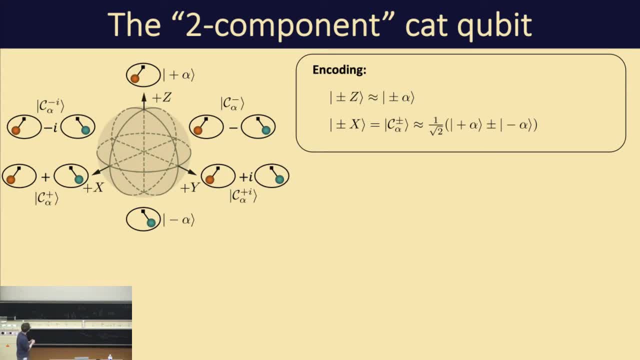 axis we have these coherent states and along the other axis we have these cat states. So these cat states are superpositions of the coherent states and for instance along the x-axis, here you have the even and odd superposition and you can work this out. It's a nice back-of-the-envelope calculation If you. 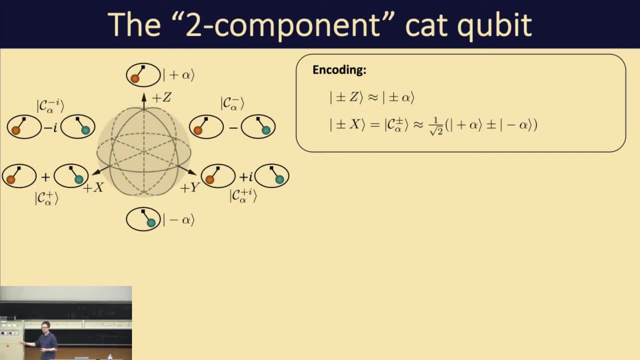 write this in the state photon number basis, you'll see that the even cat drops out all the odd photon numbers, so it has what we call even photon number parity. and the odd superposition has only odd photon numbers in it, so it has odd photon number parity. This will be important in a second to. 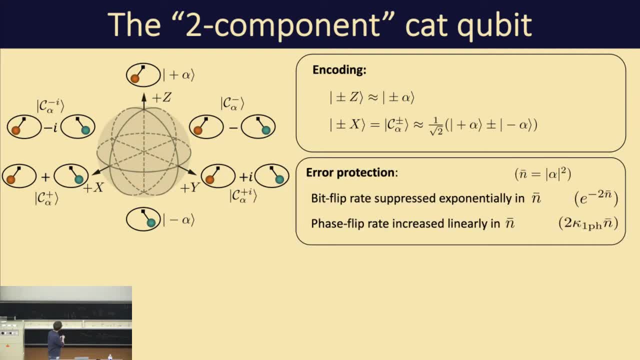 understand the error correction capabilities of this, All right. So what are the error correction capabilities? You have this notion of distance and phase-space, which also translates to a photon number. The amplitude squared of the current states is the number of photons that's involved, and you can 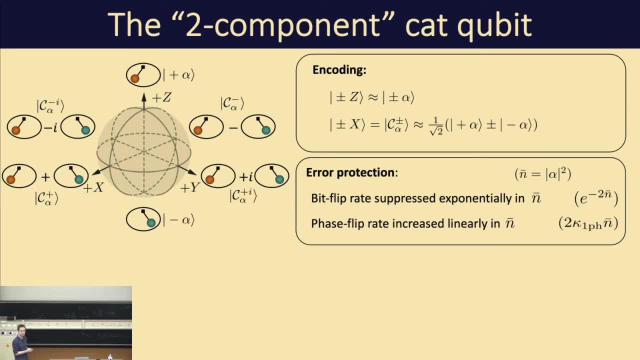 actually show that the bit-flip rate here is suppressed exponentially in that photon number. There's also a trade-off, and that trade-off is that the phase flip rate is increased linearly in the photon number. Why is that? Well, if you get one of these, 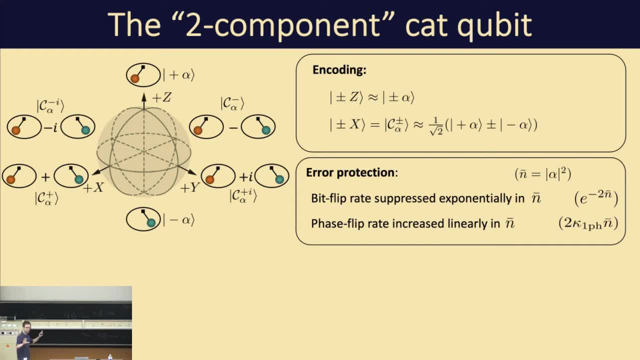 random photon jumps that you're not preventing by just repumping energy. what happens? Well, what happens, for instance, to your cat states? you're going to change the photon number- parity right, And so that flips you from one to the other. That also. 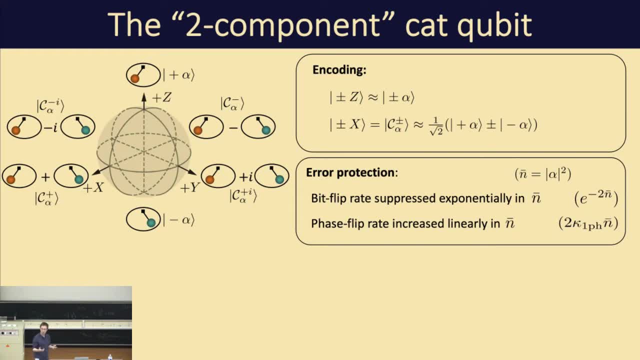 by the way, flips between the states along the y-axis, And that's going to happen at the rate of losing single photons times the number of photons that you have in your system. So you have an exponential suppression here and a linear increase here, which is 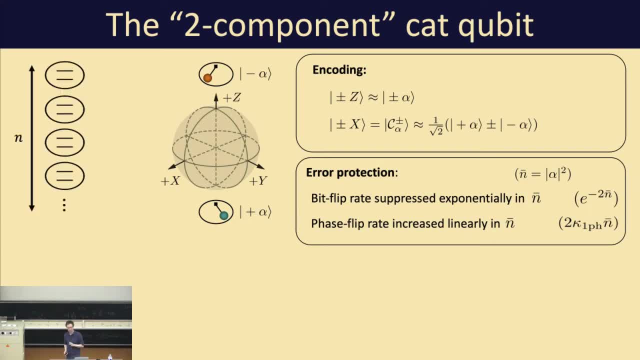 really interesting because this is actually the same way as you scale in a bit flip code, except that in the bit flip code you're exponentially suppressing the bit flip rate with the number of qubits that you're using and you're linearly increasing the phase flip rate, also in the number. 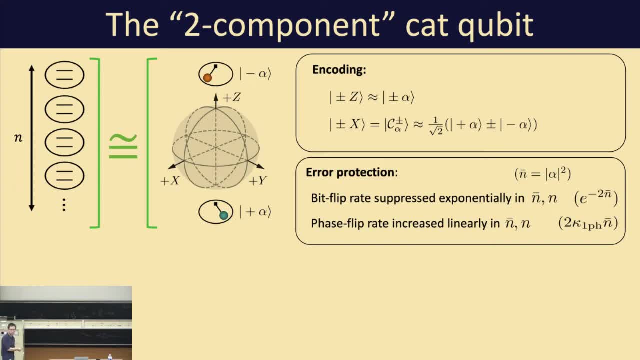 of qubits that you're using because you're not correcting for phase flips. But the crucial difference here is, of course, that the one system here uses a number of n physical systems. We're using just one physical system but n photons in that system. 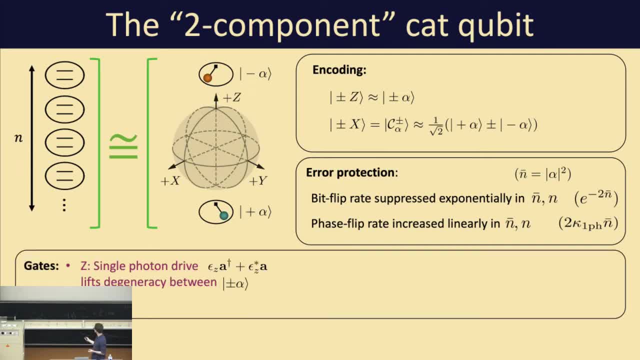 Now, this would not be useful if we couldn't do gates. In fact, you can do gates. You can do a gate around the z-axis. I will not speak in detail about those, but let me know afterwards. if you have any questions, You can do a discrete. 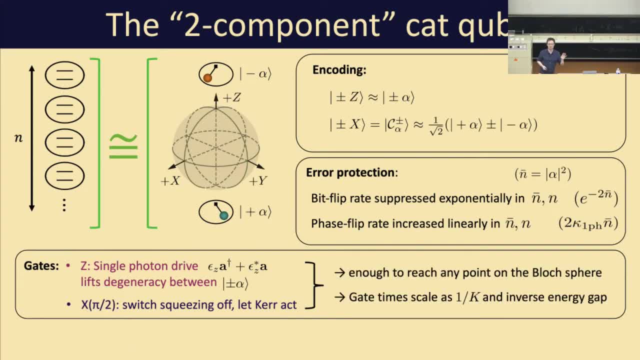 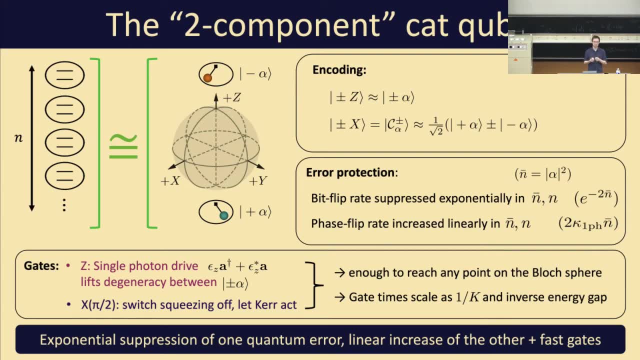 gate around the x-axis, and these are enough to reach any point on the block sphere, and they can be pretty fast. So we have here a relatively good trade-off that we can capitalize on. Now, how can you capitalize on these kind of systems? 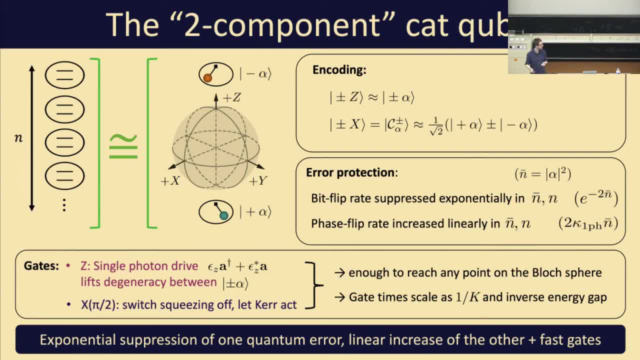 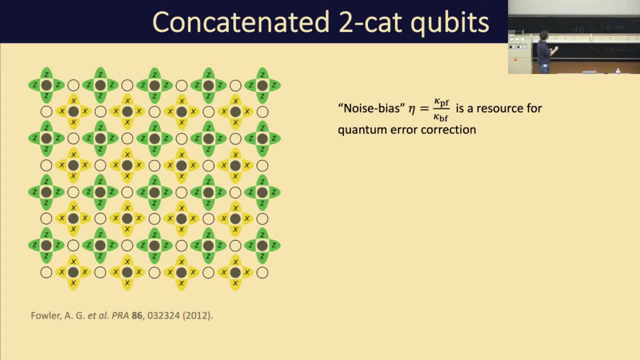 How can you actually include this in a higher order error correction paradigm? For that, let's go back to the surface code picture that we had at the beginning. What we have with this qubit is a so-called noise noise bias, So you have an imbalance between the. 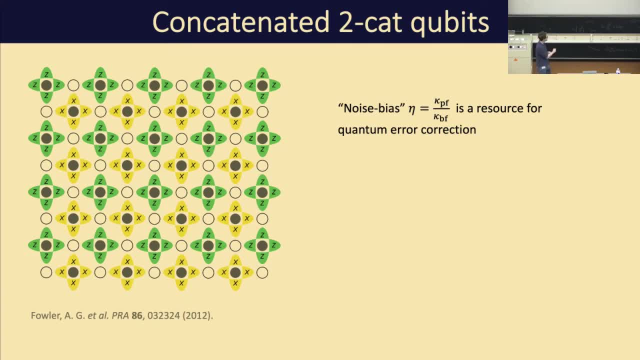 phase flip rate and the bit flip rate Okay, And that is a resource for quantum error correction and people are really realizing this more and more. Very recently, for instance, there has been a different kind of surface code that was proposed, the so-called XCZX surface. 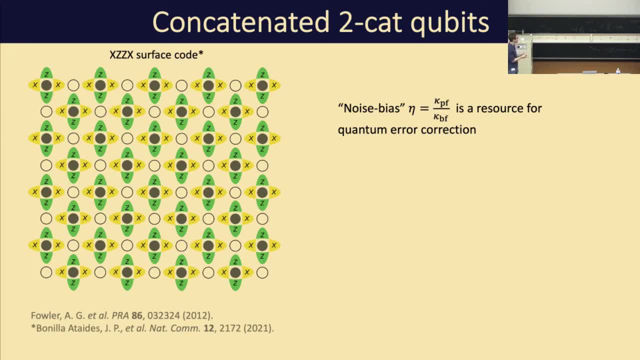 code where now, if you compare this to the other surface code that I talked about earlier, here you have these four-way correlators that are where one auxiliary qubit measures only z or only x, right In this one. it's a really small change. 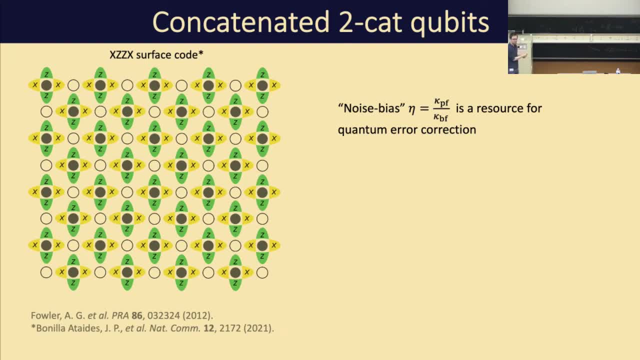 You measure instead XCZX. Now, what this allows the surface code to do is that you essentially can make use of noise bias. Let's say, your bit flip is completely gone and you only have phase flips, right, In that case you can just 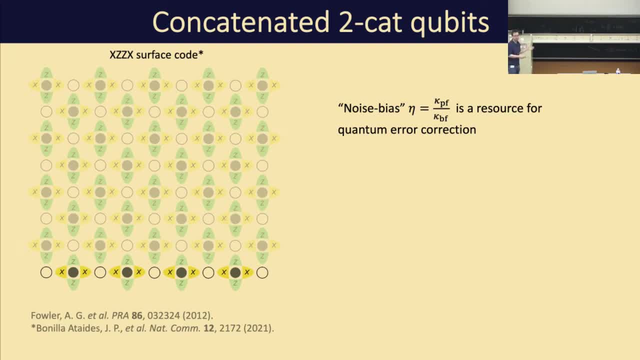 collapse the entire surface code onto one line and you do a phase flip repetition code and you're done right. Of course, experimentally we won't get rid of bit flips completely. We'll always have some bit flips, but then you just increase it. 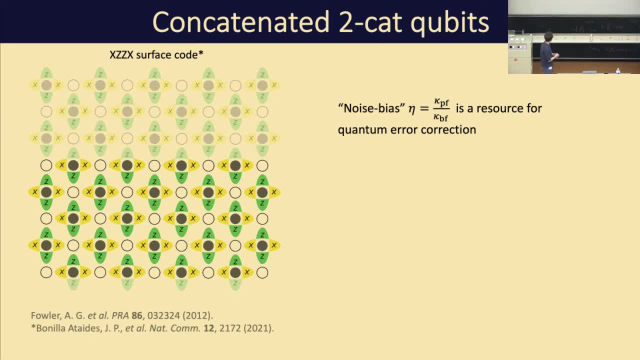 and put a bit of bit flip protection back in. Now, what people have shown in these papers is that the reduction in the number of physical system is one over the logarithm of this noise bias, and if you're not picky with the basis of your 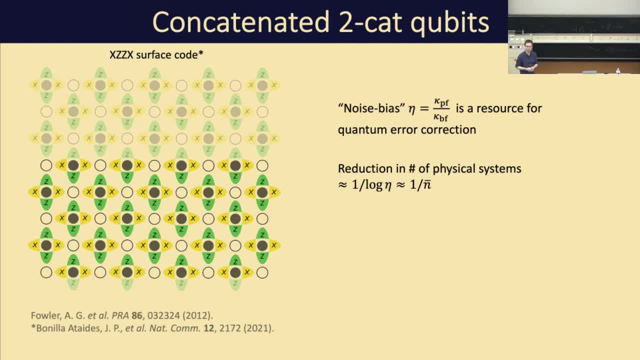 exponentials, you can say it's approximately one over the photon number in our case, And you can get further overhead reduction with bias, preserving operations that are only possible with these kind of bosonic qubits. I won't have time to talk about this here. What I 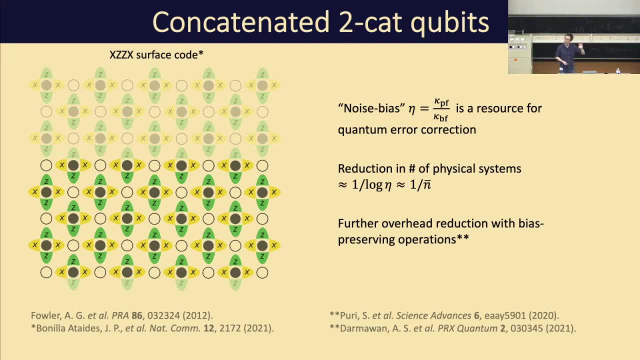 just want to give here is kind of a vision of where this could be going. Now I want to speak a bit about how such a system is implemented before moving on to a different kind of cat qubit that, in fact, can fully error correct. All right, 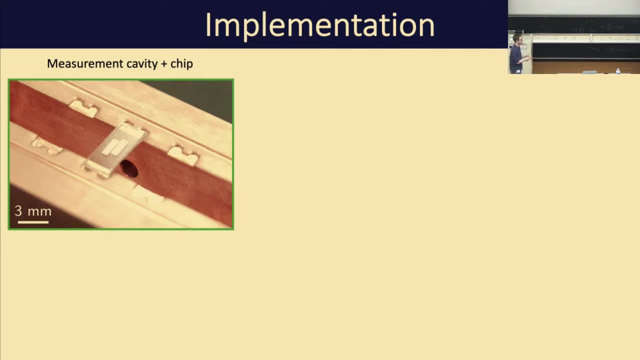 so how does such a system look like? Well, it's a superconducting circuit system. Here, what you're looking at is a 3D measurement cavity. it could be 2D. in this case it was 3D- with a chip inside. 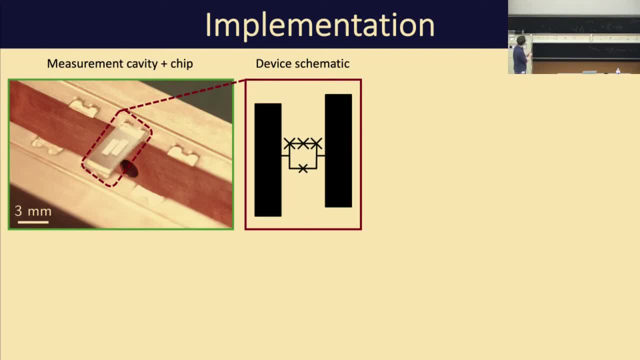 where you have two capacitive pads connected by a nonlinear element made from chosen junctions. This nonlinear inductance essentially has, you know, a bit of a more complicated structure, with three big junctions. one small junction can be threaded by a flux. Here's a zoom. 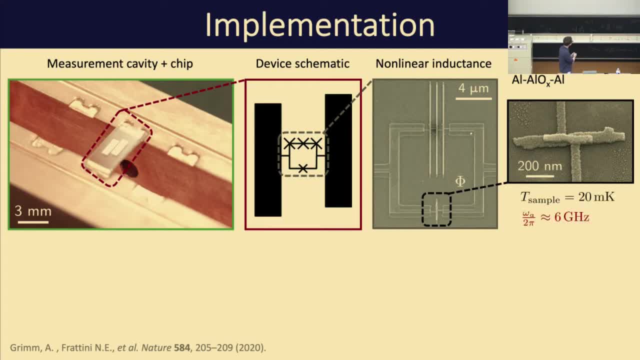 of one of these junctions and what this helps us. or I should say: yeah, of course. we operate always at, you know, millikevin temperatures, just like in standard superconducting circuits, with our samples, because our resonance frequencies are also in the gigahertz. 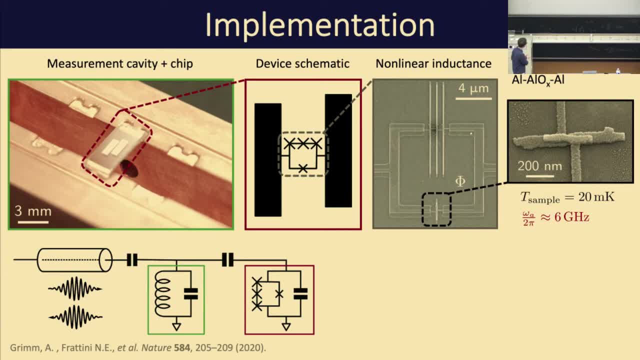 regime. Now, if you prefer a circuit diagram, that's how this would look like, where you have your nonlinear oscillator, your anharmonic oscillator, capacitively coupled to a measurement resonator, and then you have some transmission line going out of your dilution refrigerator. 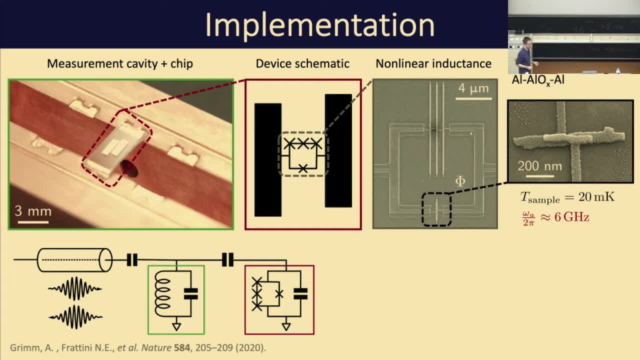 where you can send signals in or you can receive signals back. So this system is used to implement this kind of Hamiltonian, just because we can tune our nonlinearities that are present in our system very finely with these kind of circuits that we can design. 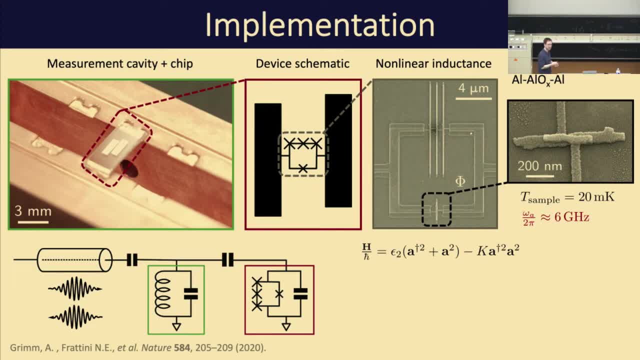 where we optimize the different sizes of the junctions and the flux biases that we apply In this specific case. we have a fourth order- nonlinearity- chi-three term for the optics community- where we mix four of these operators together in. that gives you this Kerr: nonlinearity, the. 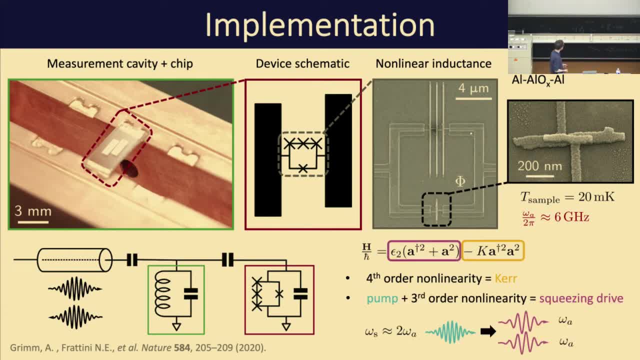 anharmonicity that you've already heard about earlier too. But we also have a third order nonlinearity, and that allows us to implement the squeezing drive, simply because third order nonlinearity means three wave mixing right, Three wave mixing means we can now apply a drive at 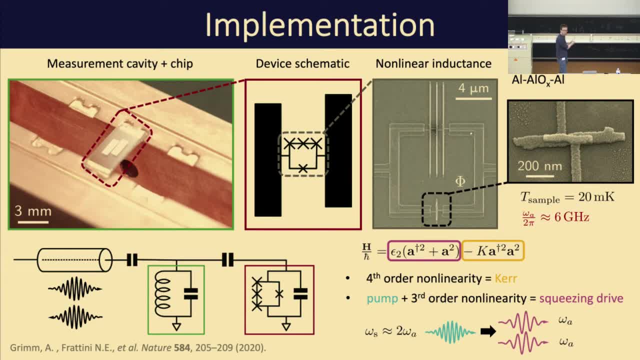 two times the frequency of this mode and then one photon on that drive can convert two photons at the frequency of the mode and voila, that gives you the squeezing drive Now doing this. in our recent experiment, where we've shown this type of 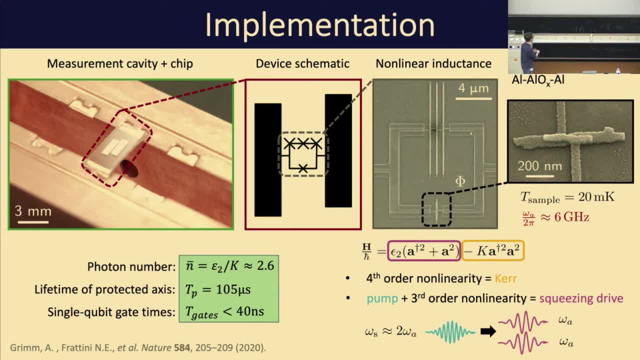 stabilization. for the first time, we have shown a photon number of 2.6,, which is modest. there's a lot of potential for getting this better, but with this already we showed that the protected axis had a lifetime of 105 microseconds, which was a marked increase. 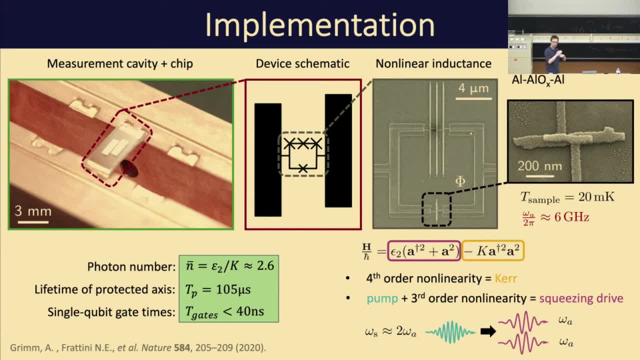 with respect to the benchmark of the just zero-one state encoding and could all do all single qubit gates in less than 40 nanoseconds, And we show the new kind of readout for the system also. so go check out our paper if you're interested. So I'm going to show you a little bit more of this now. 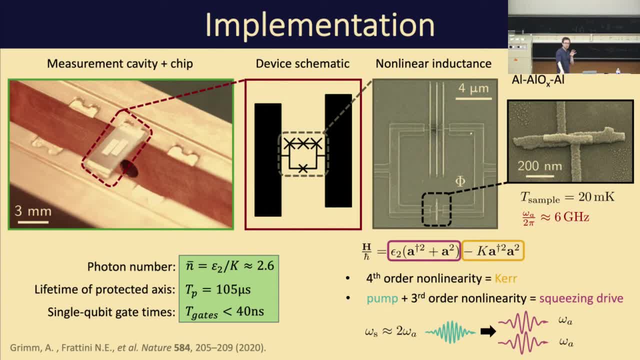 Now I want to switch this a little bit. I want to now talk about a different kind of encoding, right? So far we've talked about two-component cat states. now I want to talk about four-component cat states. What do I mean by four-component? 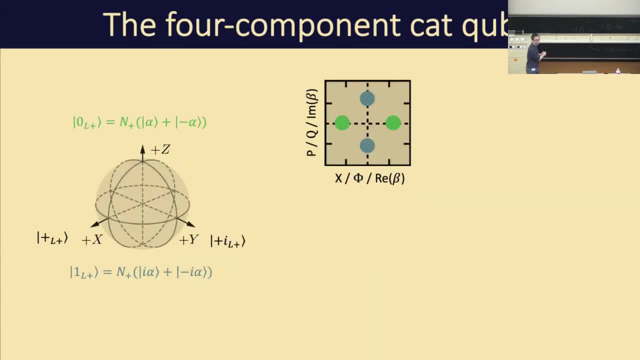 cat states. Well, you probably guessed it, I mean this: we're now going to superpose four different coherent states, And what's special about this is now, on the north pole of our Bloch sphere, we have an even photon number cat that's oriented along the real. 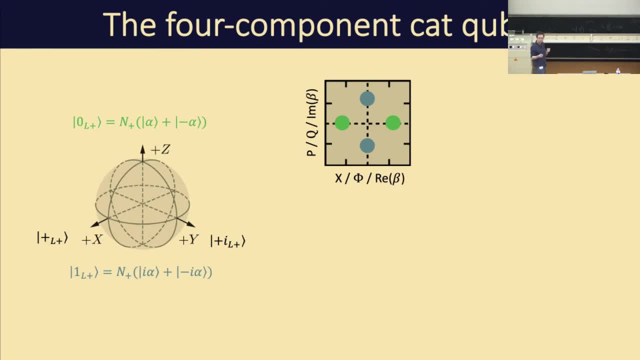 axis, and on the south pole of our Bloch sphere we have another, even photon number cat that's oriented along the imaginary axis. What does this buy us? Well, first, we don't lose anything. we still have a similar protection through the distance. 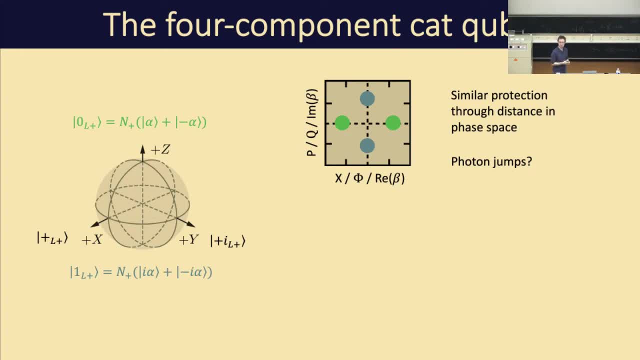 in phase space right, especially if you increase the amplitude of these states. Again there's going to be, you know, the notion of this exponential suppression of flips between these states. but now we can also deal with photon chumps. Why? 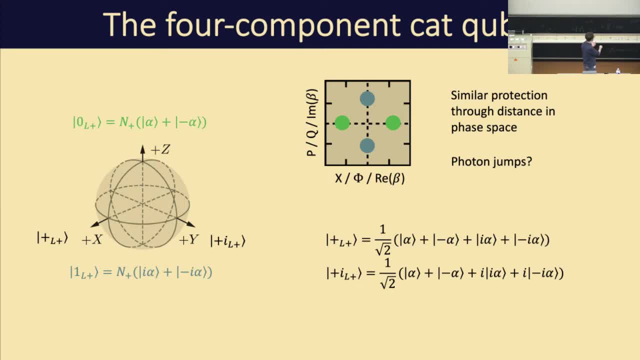 Because every state on the surface of our Bloch sphere is now made up of superpositions of even photon number states. so all the states on the Bloch sphere have even photon number, And that means that now we can detect photon chumps by measuring the photon number. 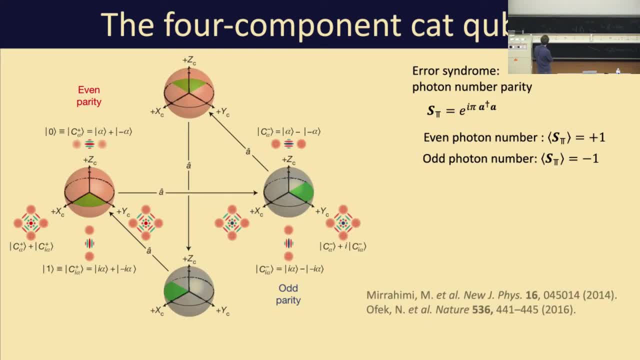 parity of our system. Now, yeah, excuse me for the small labeling. this is directly taken from a paper. How would this look like? Here's the original encoding that we had that I've shown you in the earlier picture. where these images here. 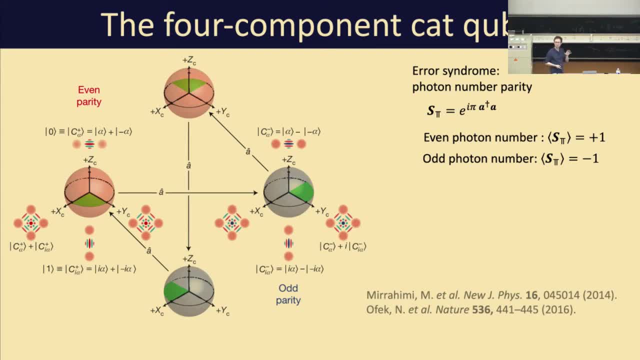 are the so-called Wigner functions. That's just a snapshot of how this looks like in phase space, where you have the two disks, the coherent states and these fringes in the middle that stand for. that show you that it's a quantum. 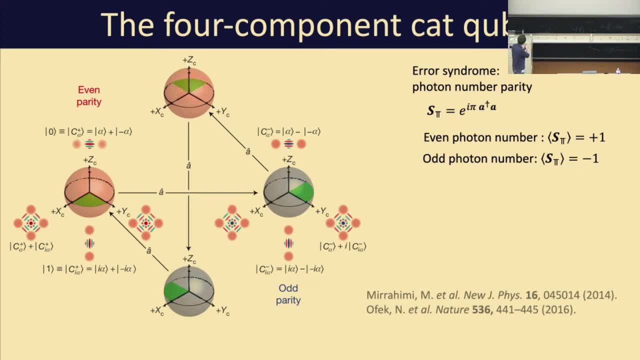 superposition, If you want to get some intuition for this. on this color scale, the center: if it's red, it shows even photon number parity. If it's blue, it shows odd photon number parity. And now, if you get a photon chump, you move entirely. 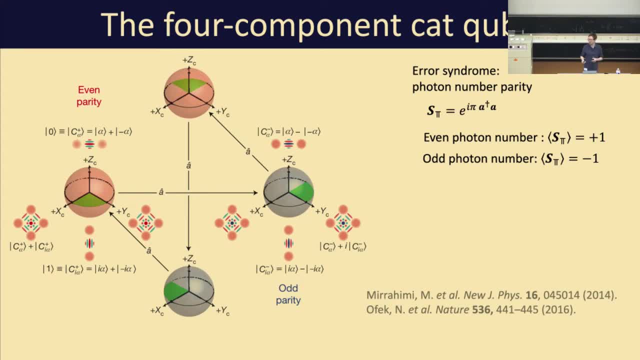 different block sphere where everything is odd: photon number parity. You also have a phase rotation indicated by this green circle segment and that's because you have an imaginary unit in there also. So that's also a nice back of the envelope calculation to do to check that. 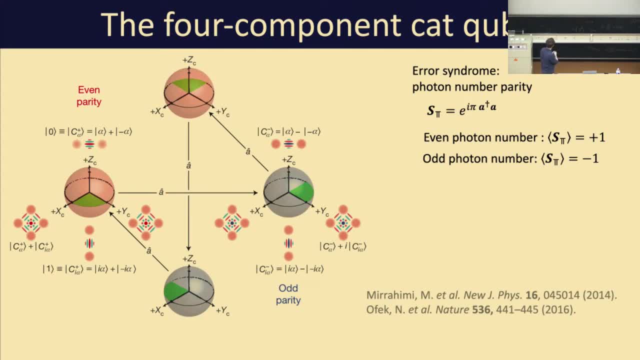 it really chumps between these blocks sphere. If you then have another photon chump, you go to another even parity block sphere, another odd one and you come back to the same even parity block sphere. So you keep going around like that And that means we can now measure. 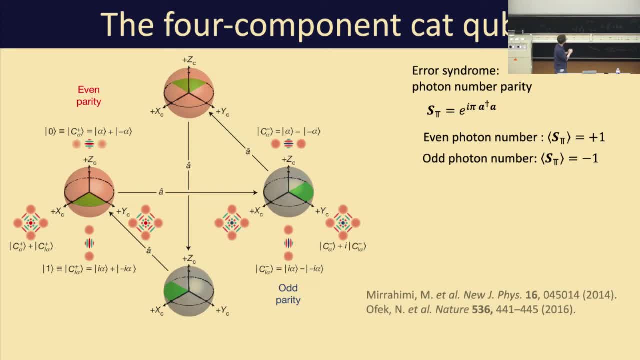 this error syndrome, this photon number parity operator, which is given by this expression, where the expectation value of this operator, for even photon numbers, is going to be plus one and for odd photon numbers it's going to be minus one. So, in principle, by just tracking these, 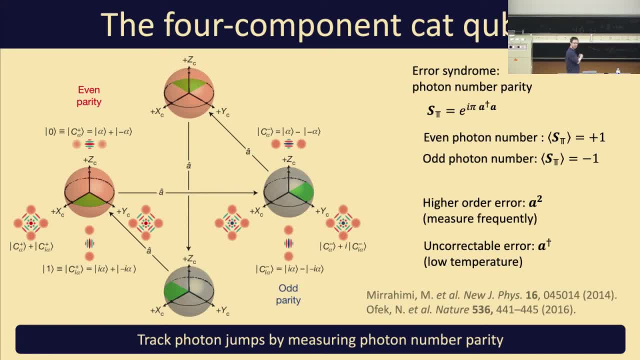 photon chumps. we can exactly know what happened to our quantum information. We don't even have to do an uncove, a redo or recovery operation, We just follow it and know what happened. right, There are some caveats. For instance, you can get: 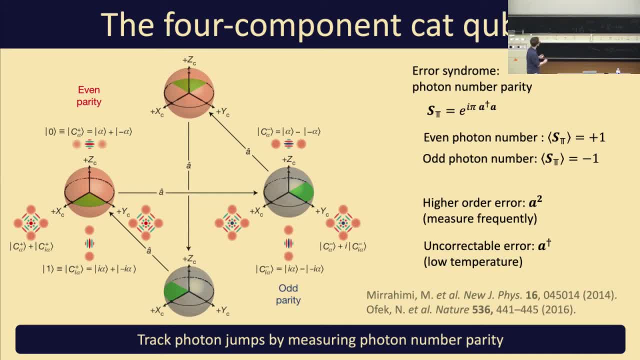 higher order errors. right, Higher order errors are going to happen if you get two photon chumps in between parity measurements. These can of course be compensated for by measuring the parity faster and faster, but experimentally you always run into a limit here And then. 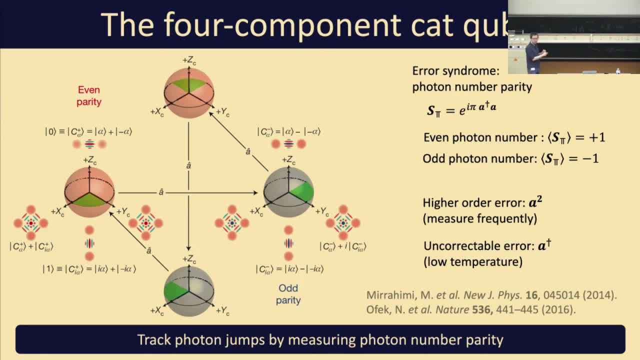 there are uncorrectable errors. What's an uncorrectable error? Well, let's say you gain a photon in this paradigm, right, Then you're not going here, but you're going here and you see that there has been a change in photon number: parity. 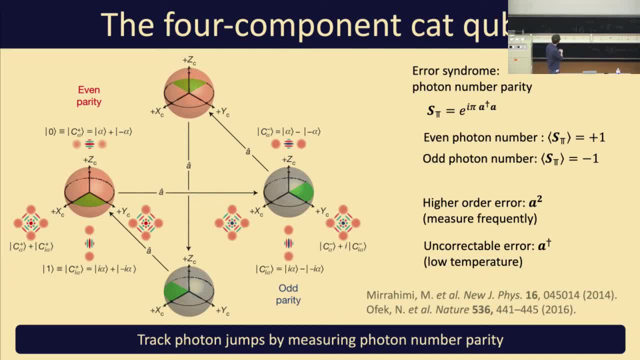 But of course you're thinking that you're here and so you're not correcting for the right thing. So that is luckily something that happens rarely in superconducting circuits, at least with resonators in superconducting circuits, because the low temperature that our 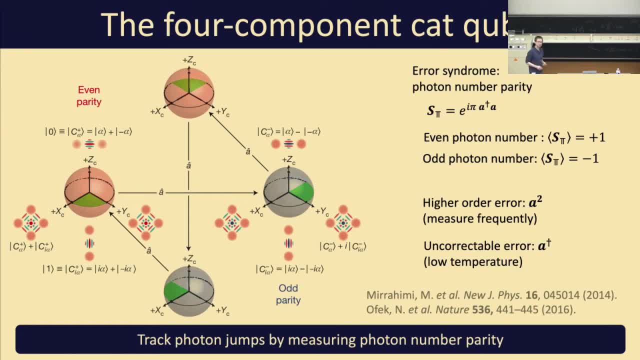 experiments are run at guarantee that we're in a pretty low thermal population number of the excited state, which dictates how often these up jumps are going to happen. Okay, so how does such an experiment actually look like? This is now a little bit of a different. 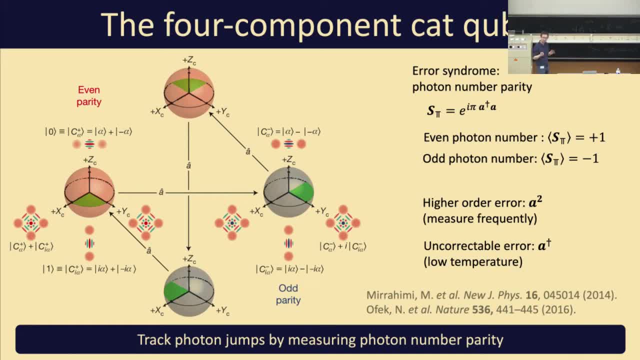 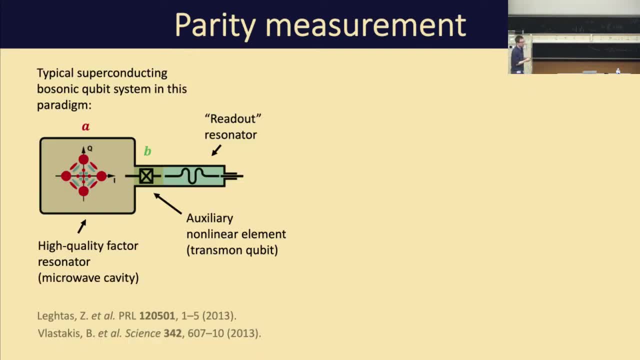 architecture than the one we saw earlier. Earlier we encoded into an anharmonic oscillator. Now we're going to use a combination between a harmonic oscillator and a nonlinear system. So the standard approach for this kind of four-component cat is: you have a high-quality factor resonator, a. 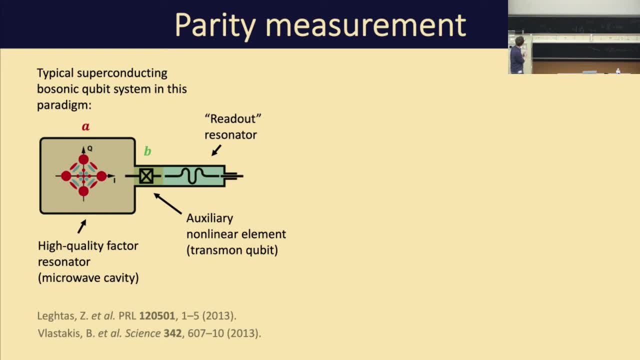 microwave cavity. that's why it's this weird enclosure here. and then you couple that with an auxiliary nonlinear element, which very often is just a transmon qubit, right, And that will give you the nonlinearity that you need to make interesting quantum states in the 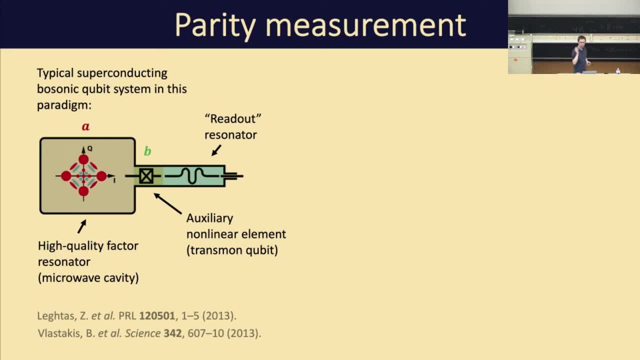 harmonic oscillator that by itself, otherwise would be pretty boring. All you can do is drive it and you get a coherent state right. And then there's also a readout resonator. we talked about this this morning, I will not talk about. 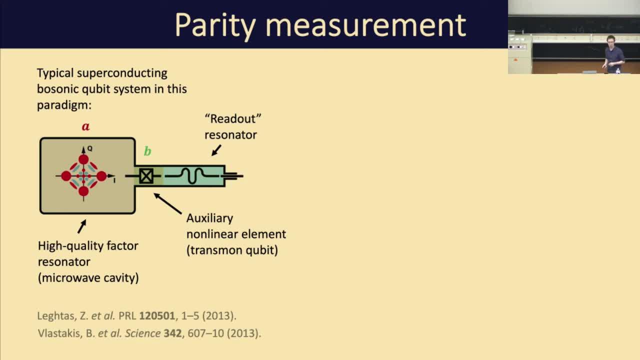 this a lot, but it's essentially just here to then measure what state the qubit is in. Here's the Hamiltonian for the system. You've also seen this this morning, So you have a frequency term coming from the microwave cavity. You. 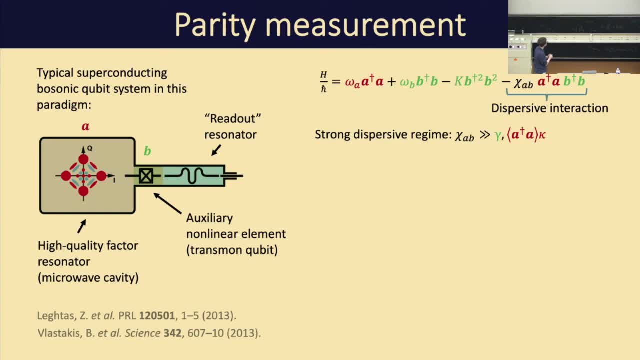 have a frequency term coming from your, from the qubit, and the non-linearity of the qubit, and we are in this regime that Christopher has shown you, where we have dispersive interaction, where the frequency of one of the systems gets shifted based on how many excitations you have in the other system. We are additionally in the 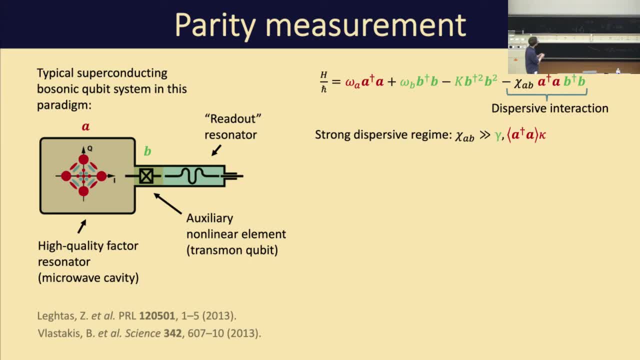 strong dispersive regime where in the line width of the cavity- and additionally, our requirement is going to be that the average photon number of the cavity times the line width of the cavity is also smaller than this dispersive interaction because the- if you remember the two cat example- 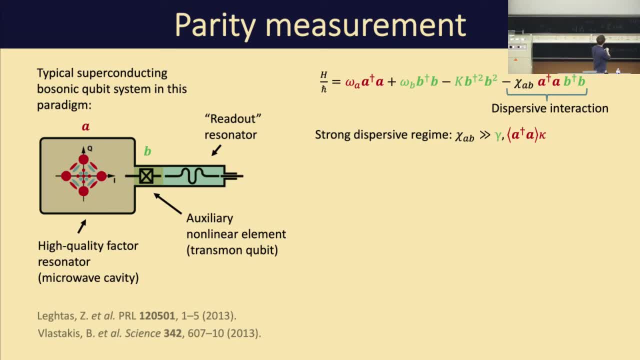 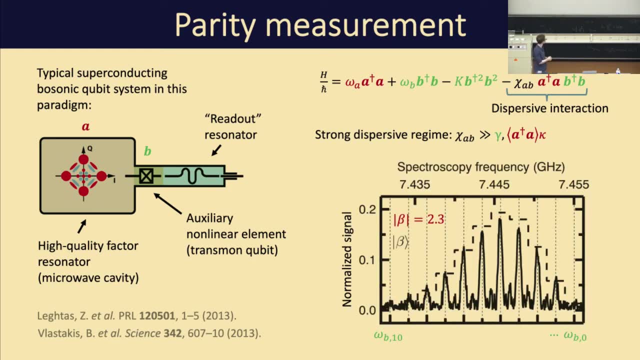 the coherence of these states is going to decay at a rate that is the average photon number times the line width right. So just to show you how such a system experimentally can perform. so this is taken from this paper here. this is spectroscopy of the qubit g each. 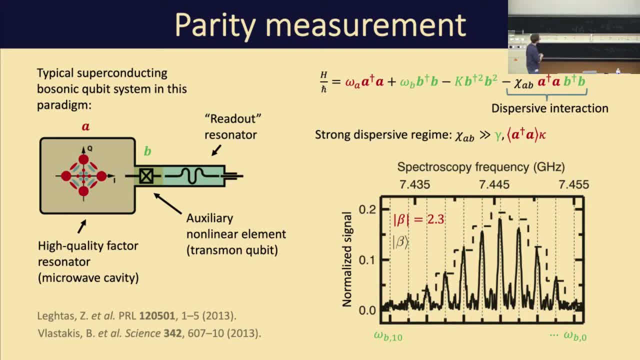 transition as a function of frequency if the cavity is prepared in a coherent state with 2.3 photons in it. So here you see, this forest of peaks, and that's really. you're trying to pulse the qubit from g to e and it has now different frequencies depending on each photon number. that 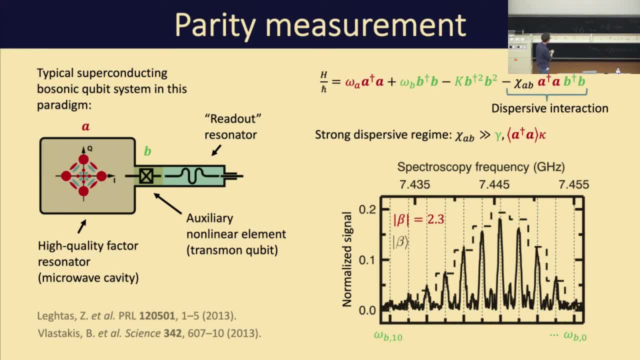 is in the cavity right, This is a Poisson distribution and you can actually see this little stairwell here shows the ideal Poisson distribution. So you really see, for no photons in the cavity. You have this transition frequency for one, this and so on, and goes to 10 and that actually gives you a way to really measure the photon. 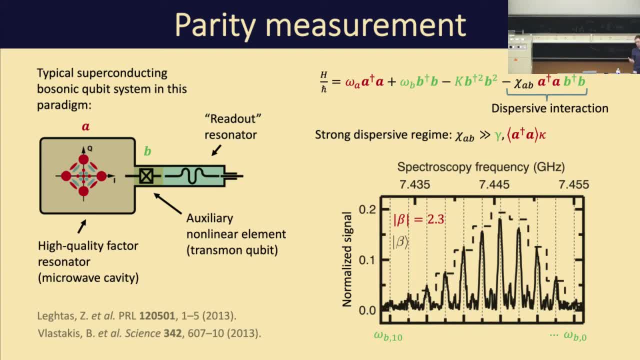 statistics that you have in your cavity, and in principle that already would be enough to measure the parity, which is how we measure the error syndromes. But here you of course averaging over many experiments. what we want to do is to measure the parity in a single shot, and that's also. 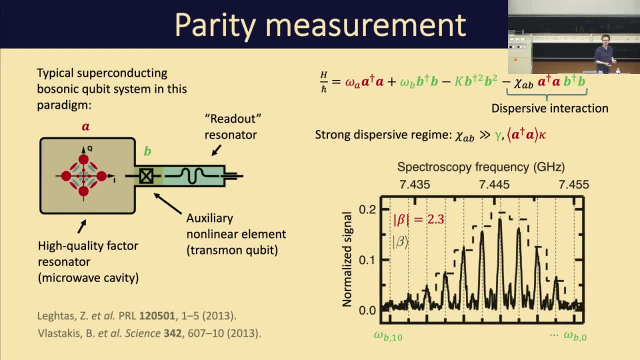 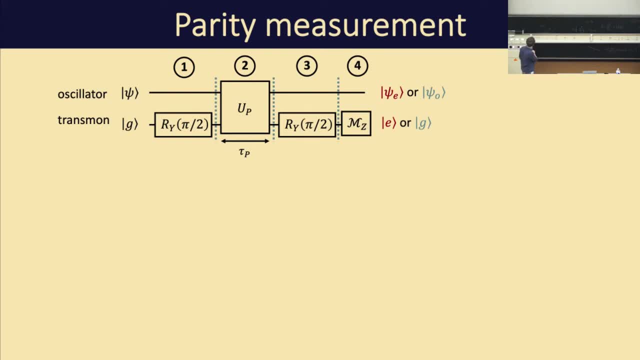 possible And I wanted to give you an idea how such a measurement can be implemented in practice. So that's the sequence for such a measurement Here we have two timelines: an oscillator and the transplant of the oscillators. the cavity, or if I use these terms interchangeably, and the cavity is in the in some. 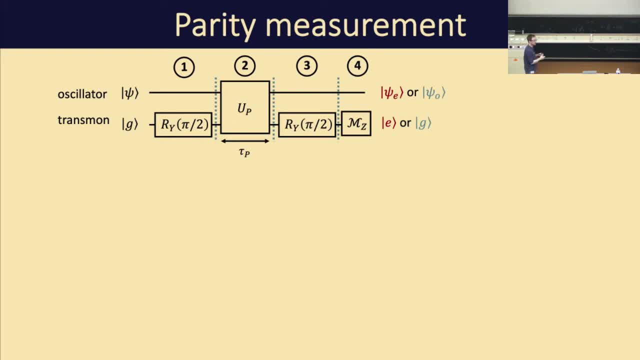 state sigh at the beginning and then the transplant is going to be in some in the ground state essentially, If you're reading from left to right here. so there's four parts and I'll just walk you through these four parts. We start out with the transplant in G and we do a pi or two pulse around the y axis on it, which 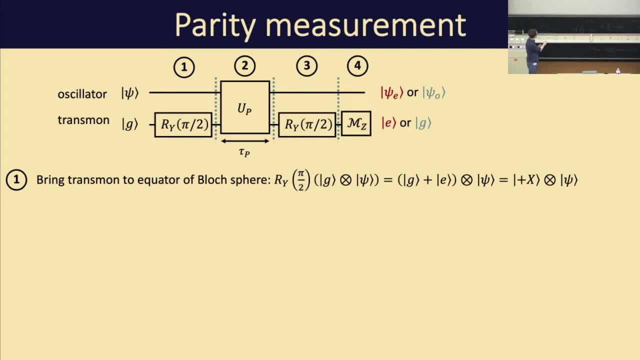 brings the joint state between the transform and the cavity G tends to product Psi to G, plus E Psi or plus X Psi. So far, that's nothing special. Then the next step is the crucial one. There we make use of this interaction, this dispersive 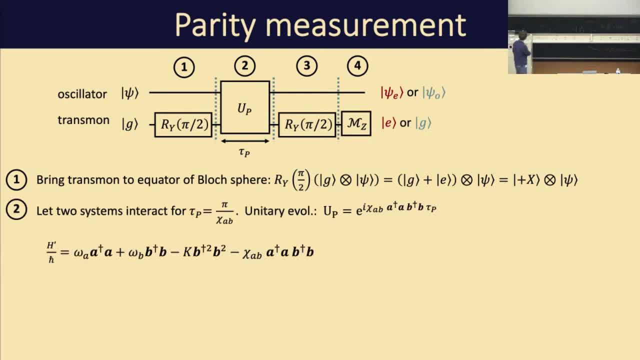 interaction between the two systems, where we let them interact for a given time. pi over KAB- I'll get back to that- and that corresponds to a unitary revolution given by this operator here. Why am I picking that? Well, that was our original Hamiltonian and here I've just gone. 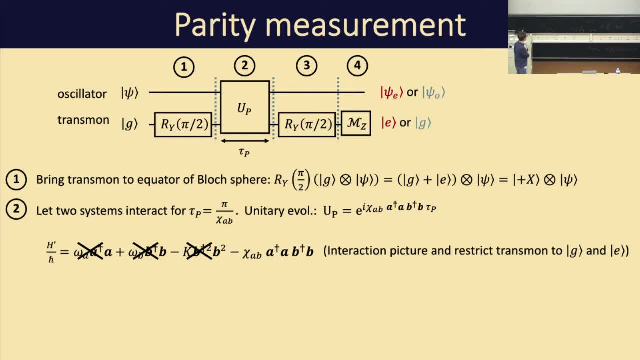 into the interaction picture with respect to the frequencies of the modes. and I've also eliminated this non-linearity because we're just restricting the transform to the G and E levels, where it doesn't play a role. So that's our Hamiltonian and here we've just exponentiated that We can write. 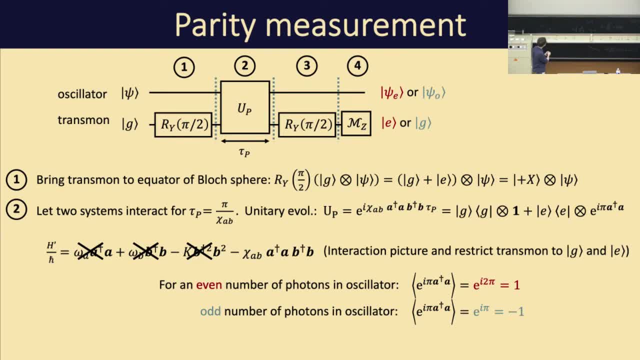 this in terms of projectors, right? So what happens if the transform qubit is in the zero state, and this here is one? so we have the G tends to product projector and then if it's in the one state, then you just get this. 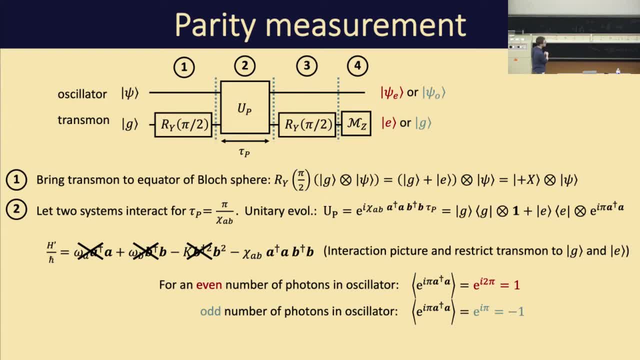 This operator here, where pi is the only thing that survives because of the time that we've chosen. And then you get the E projector times, this parity operator that we were looking for, And this, of course, as I mentioned earlier, is going to be one for an even number of photons. 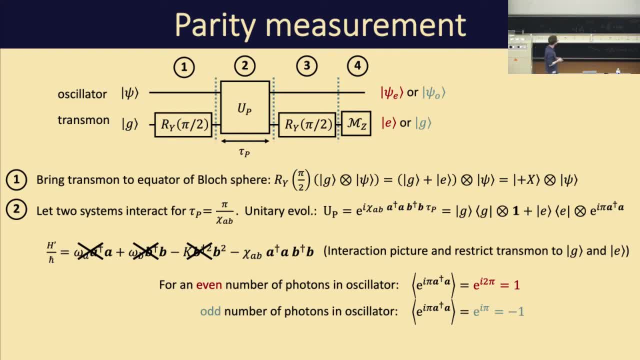 in the oscillator and minus one for an odd number of photons in the oscillator. So after this evolution we end up with an entangled state where if you had an even number of photons in the oscillator, then the transform is still in plus X, but if you had an odd number of photons in the oscillator, 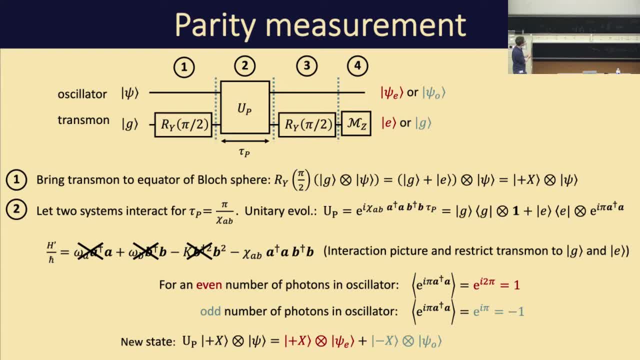 then you've picked up a factor minus one in the E state and it's going to be in minus X. This equivalently also is going to just slice out the superposition of even photon numbers or odd photon numbers from an original state, psi, and that is actually useful for creating cat states. 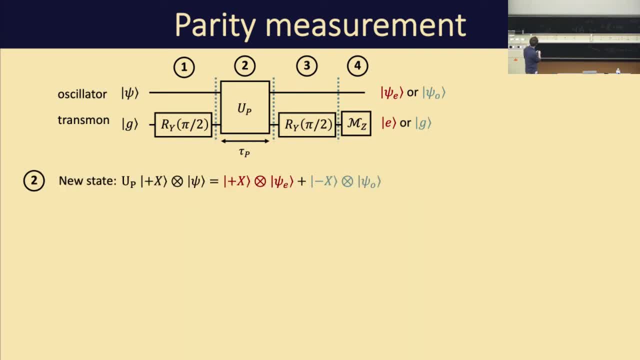 Now let's put this up here, and we're continuing with the rest of the sequence. We're doing another pi over 2 pulse around the Y axis and that just brings us from plus X to E and from minus X to G. So now we're here. 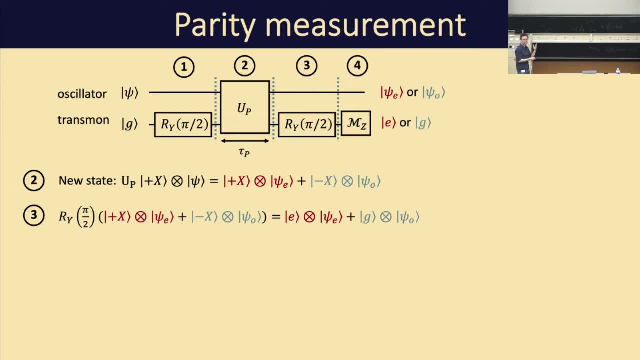 Here we're just creating this entangled state because we can only read out easily along the z-axis, which we're doing now. and then you project into e or g. You get the measurement result: e if you were in even parity state or g if you were in an odd parity state. 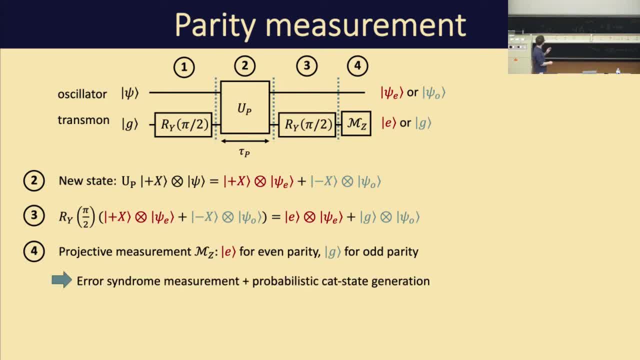 and that's how you measure this error syndrome. As I said, this can be used for more right. You can also create cat states with this. probabilistically, You just displace your oscillator, You have a coherent state. Then you do this measurement. 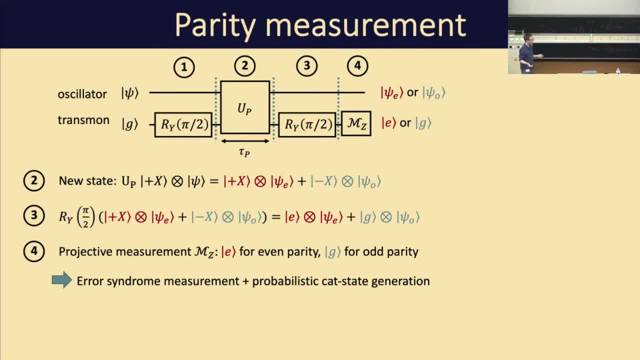 and you project at the end and you'll end up in an even or odd cat. You can also fully characterize the density matrix of the oscillator with something called the Wigner function. I'm just giving you the expression for this here. that also depends on a parity measurement. 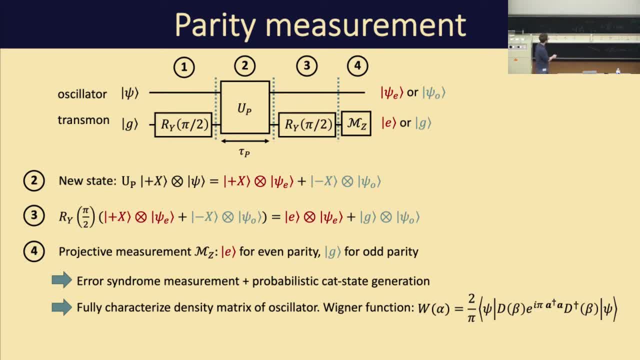 like the one I've just described, and displacements, which are relatively easy to do on these oscillators. And then, finally, a similar protocol exists for deterministically creating cat states and also perform gates on them, where the time requirement is always set by the inverse of this. 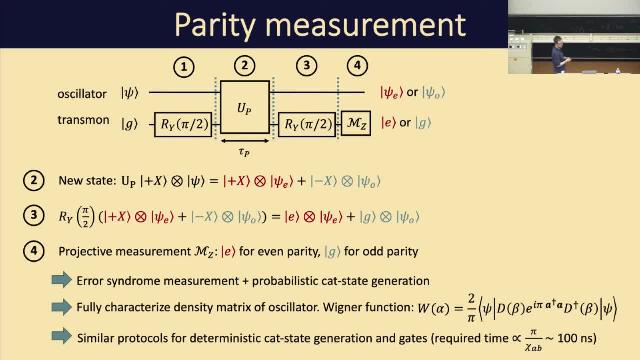 this dispersive interaction strength, So it's on the order of 100 nanoseconds or so. Now, how are these systems actually? yes, So you're just trying to correct this with the state in the cavity. That's right. With the qubit. 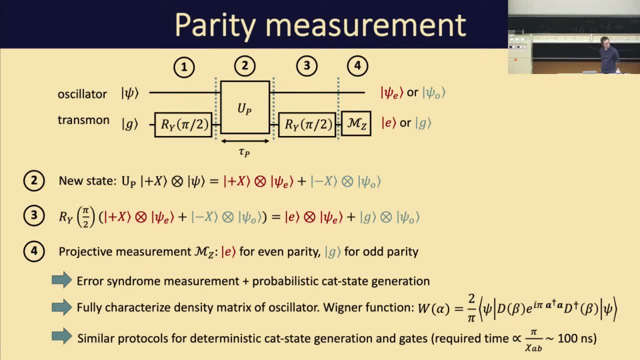 That's right. And so how, with the qubit on the object, how much does this limit you? That's yeah, absolutely So. the qubit will have, for instance, a finite state, excited state, population right, which then changes the frequency of the cavity. 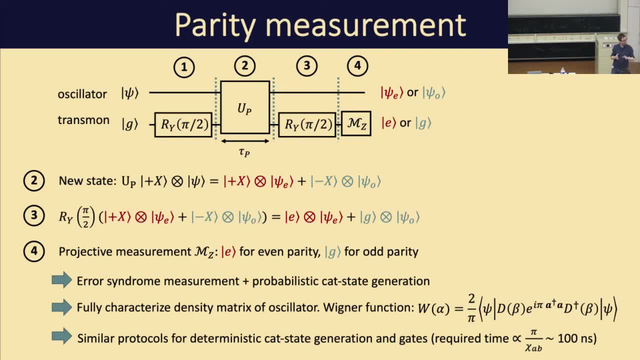 and introduces defacing on the cavity, And that is in fact a big limitation for this. but it can be circumvented And you can go see Francesco's poster, who is going to talk exactly about this, because that's what his project is on. 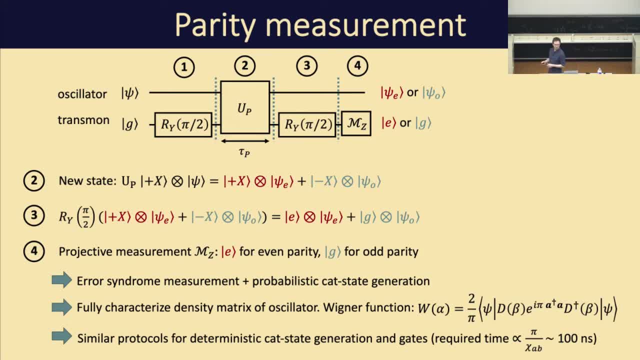 I'll come back to that a little bit at the end also. All right, so, physically, how are these systems implemented? Well, no, this stopped working. Oh, because it's the wrong pointer. huh, Oh, there we go. 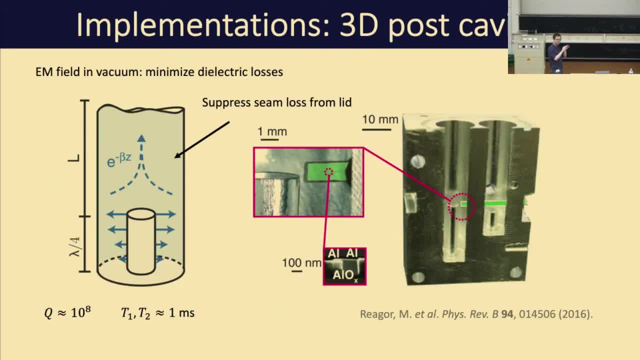 How are these systems implemented? Well, you've seen earlier that microwave resonators and superconducting circuits can be implemented with these coplanar waveguides. But these coplanar waveguides are sitting on a substrate and that substrate is a dielectric which has losses. 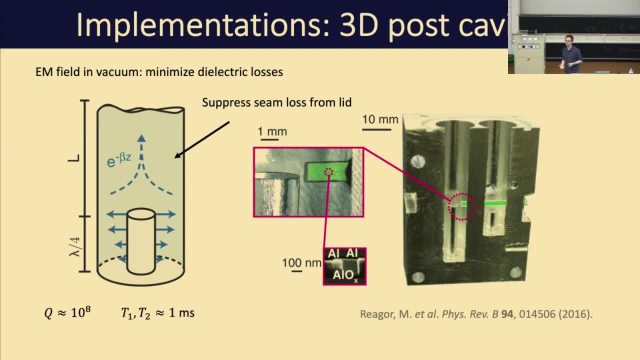 If there's a lot of field in that dielectric, then you're going to limit your relaxation time, which is why, in general, people in this bosonic qubit field like to use 3D resonators where the electromagnetic field is in vacuum. 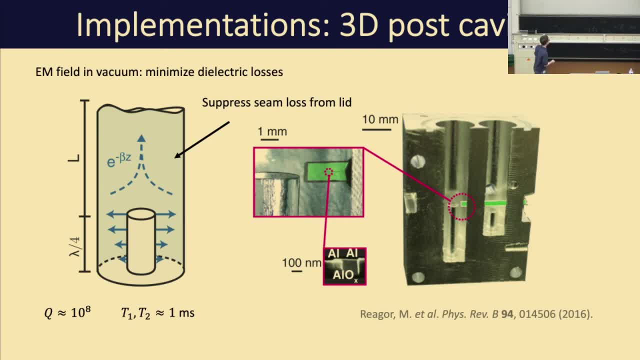 which then minimizes that kind of losses- And the flagship resonators. the resonator that's used is this 3D post cavity, So think of this as an empty aluminum cylinder that's been machined out of high-purity aluminum, And then you have a post sticking up here. 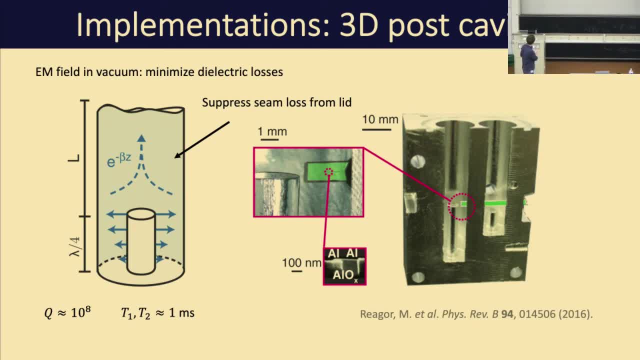 and that post has a certain length and it will resonate as a lambda over 4 resonator where the electric field is maximum up here because it's an open and minimum down here because it's a short. And the reason why people use this. 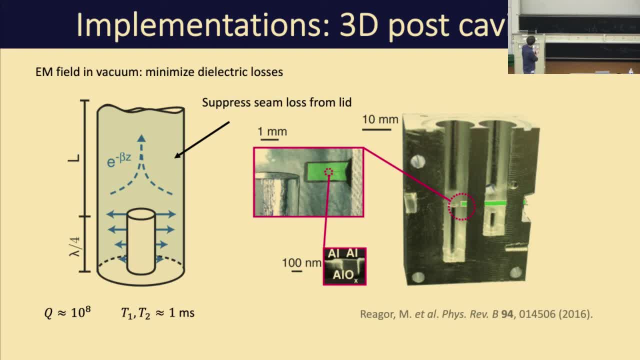 is that the diameter of this cylinder is smaller than the wavelength of this fundamental mode, and so the mode is evanescent in the Z direction, meaning that you can put the lid. the lid will include a seam that also introduces losses all the way at the top. 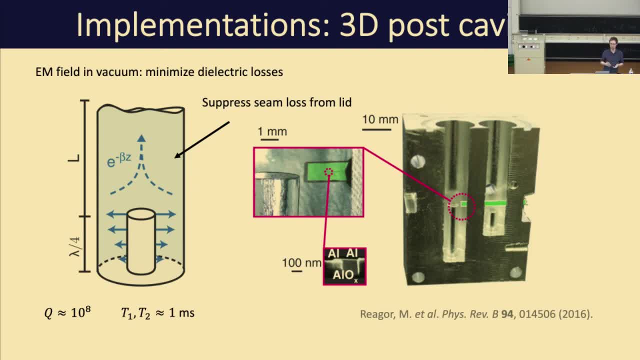 and that way you get rid of the seam losses. It's as if you had a perfect enclosure. In order to couple a qubit to this, what you do is you drill a hole into the side and you stick a chip in there with a qubit on it. 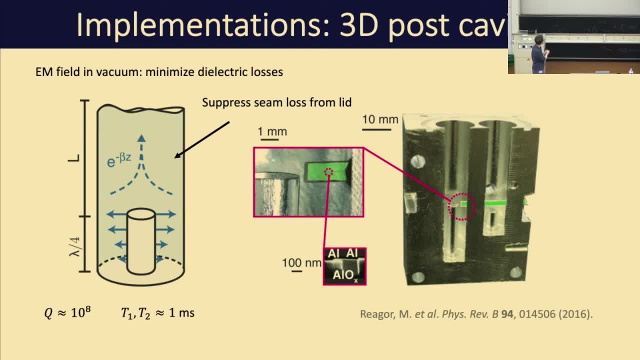 So that's, you know, some aluminum oxide junction device with some pads that couples to one of these posts and goes through the second. so here you have a cut through one of these, where that will be a high Q mode and that's a strongly coupled low Q mode. 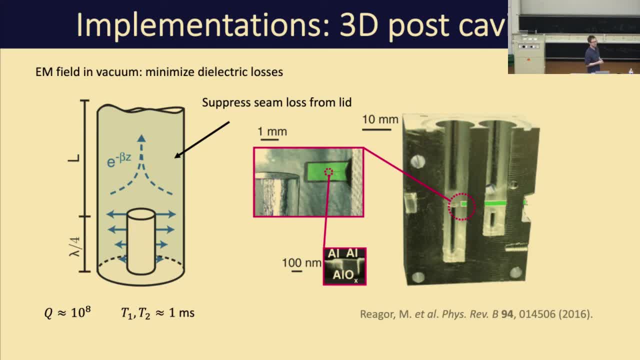 And the lifetimes and coherence times- T2 times that people achieve for these modes are on the order of a millisecond And I should mention there has been a really interesting experiment. so these are really the systems that are being used for most. 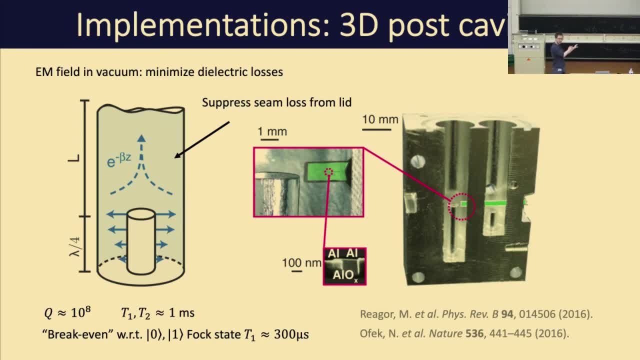 atomic quantum error correction experiments, except for the anharmonic oscillator ones that I mentioned earlier, where in this experiment they'd use the forecast, but of course they were using a highly high frequency and I should say they were using a very high frequency. 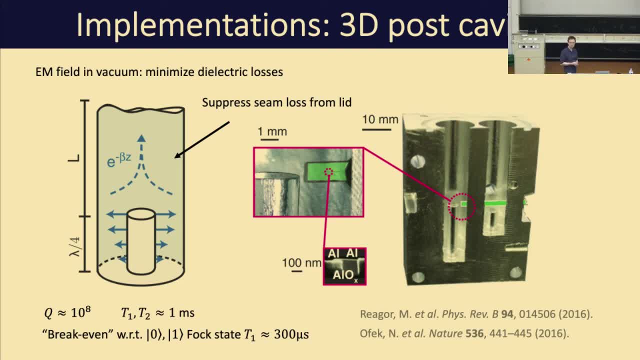 and they were using a very high frequency to be able to do that. And so the first thing that they can do is to use a very high frequency, and then they can do it in a very high frequency, and then they can do it in a very high frequency. 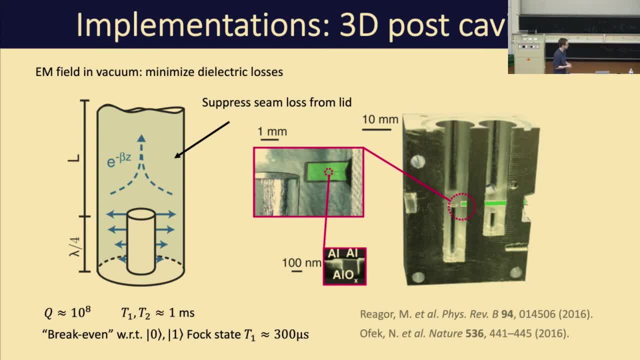 and then they can do it in a very high frequency. or at least it was operated at break even, to qualify that statement a little bit. So that's nice. but of course now you will say: well, you know, we're talking about hardware efficiency here. 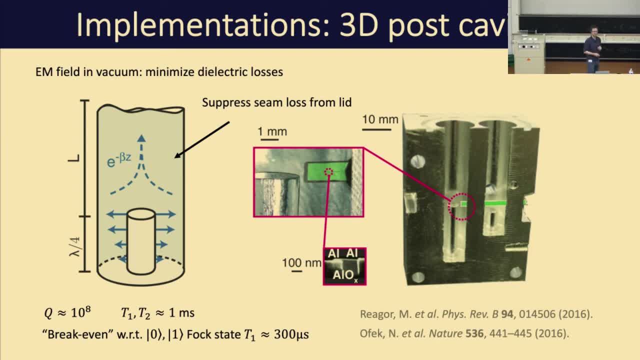 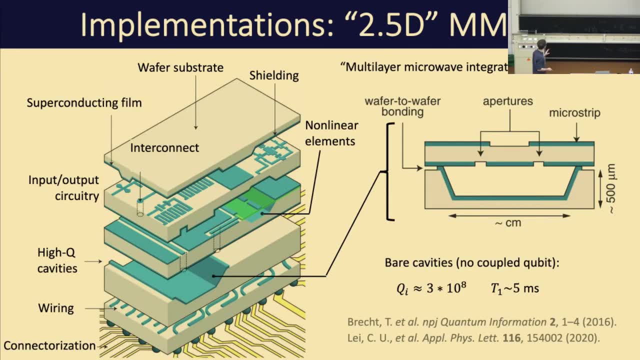 and this thing is gigantic. right, You can see that it's several centimeters in each direction, And, of course, that is something that people are thinking very hard about, and I'd like to show you quickly one of the possible solutions to this that they have come up with. 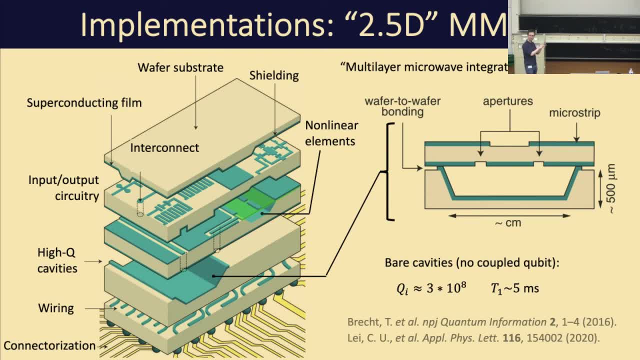 So even if you say you have many photons in your oscillator and you you know you're replacing potentially many two-level system qubits, you still want it to be as small as possible, and that's why people have invented this multi-layer microwave. 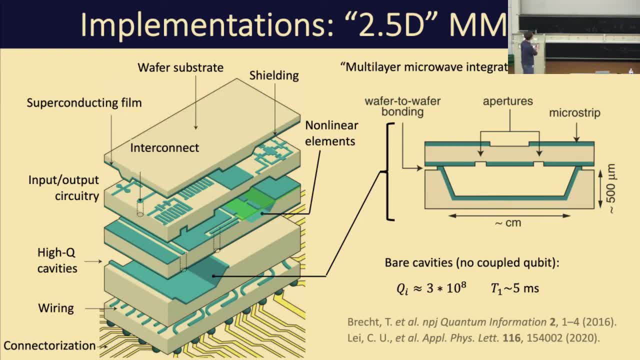 integrated quantum circuit or MIMIC or 2.5D architecture, where essentially you take many wafers that are, let's say, five, 100 micrometers to a millimeter thick and you machine out enclosures of these wafers. 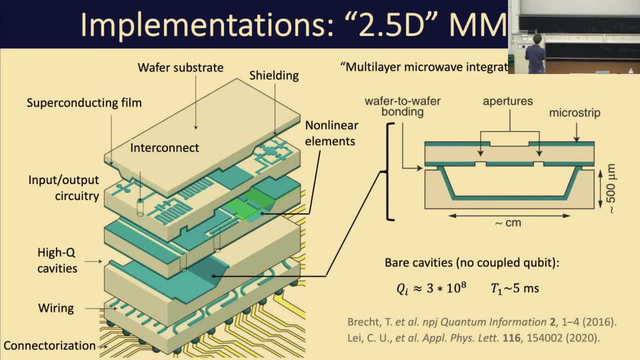 cover that with superconducting material and then you stick them on top of each other. Then you can have space for input-output circuitry, nonlinear elements, high-q cavities, wiring and so on. So it's really this stack of different. 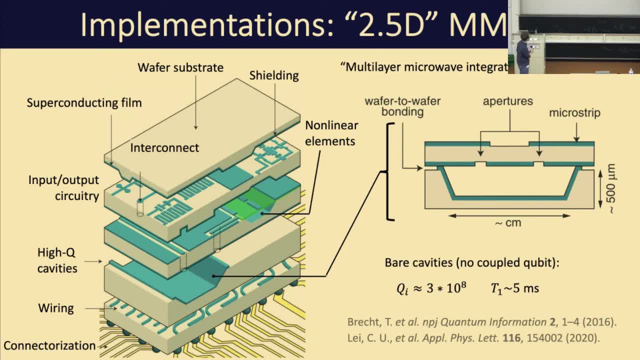 enclosures that have been machined out of wafers. Out of all this, the only thing that has been experimentally demonstrated are the high-q cavities that now have lateral dimensions still on the 10-millimeter scale or so. 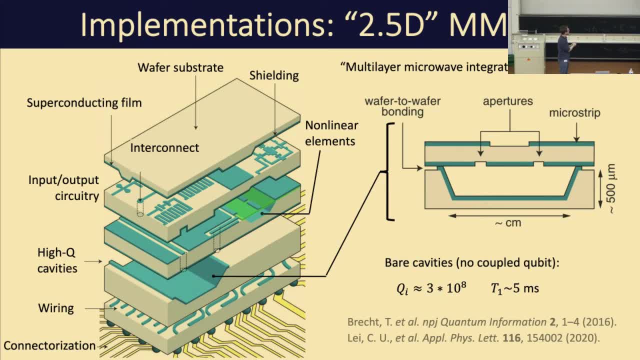 but actually have a z-direction of 500 micrometer, And that these cavities, the bare cavities, without a couple of qubits so far, have actually achieved really impressive lifetimes. So the quality factors are on the order of 300 million. 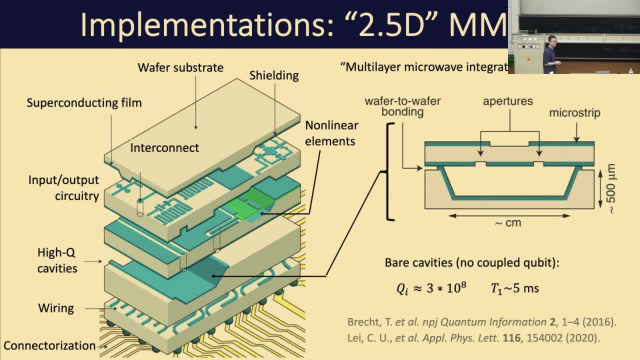 and you get lifetimes of about five milliseconds at the single photon level. So that is maybe one direction that this subfield of quantum error correction is going to evolve into. With that I have reached basically the end of my talk, so I'll give you. 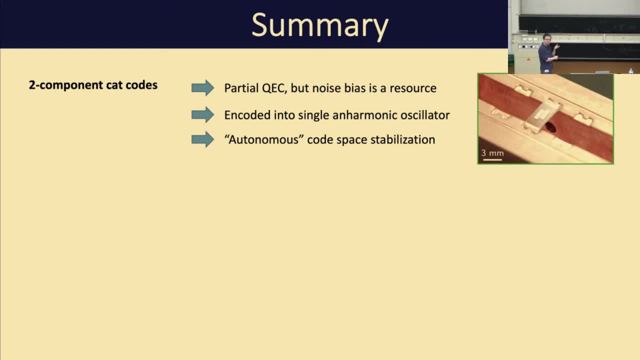 a quick summary. I've talked to you about different paradigms in bosonic quantum error correction, the two-component CAC codes, where you can do partial quantum error correction, but this noise bias can be a big resource. I've talked about how these are encoded. 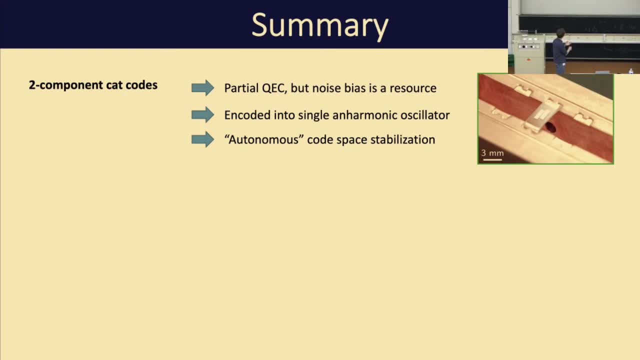 in a single anharmonic oscillator, so pretty efficient, We can autonomously stabilize the code space. and by autonomous in this context I mean we are coming up with some kind of effective dynamic that really pins these coherent states and all their superpositions in place. 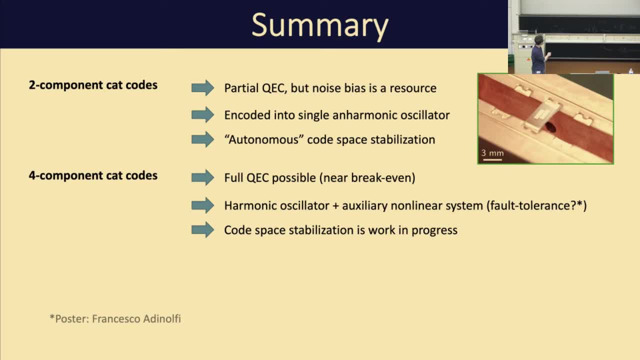 In contrast to that, these four-component CAC codes, they can fully quantum error correct and they have been near break-even. They're based on combined systems, generally with harmonic oscillator and the auxiliary nonlinear system, and that actually raises some questions with respect to fault tolerance. 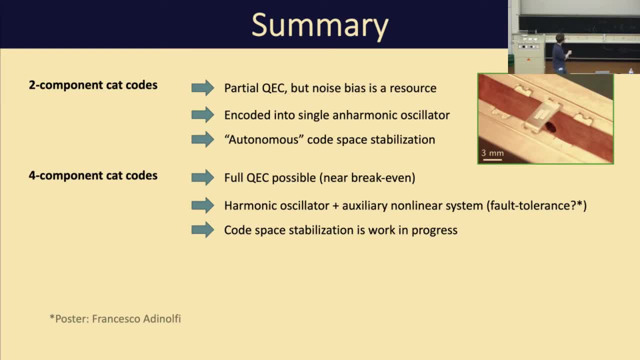 as you pointed out, where errors from this auxiliary nonlinear system, a trans one, could potentially feed back into the harmonic oscillator, into the positional system. And to avoid that you have to play some tricks and, as I said, go check out Francesco's poster. 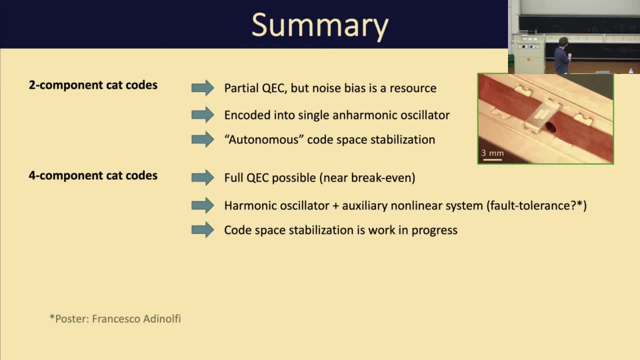 if you're interested or ask me also about it. And then the code space stabilization for this. that is still very much work in progress because it requires high order nonlinearities or other tricks. I'm also happy to tell you more about that Here. I just want to say 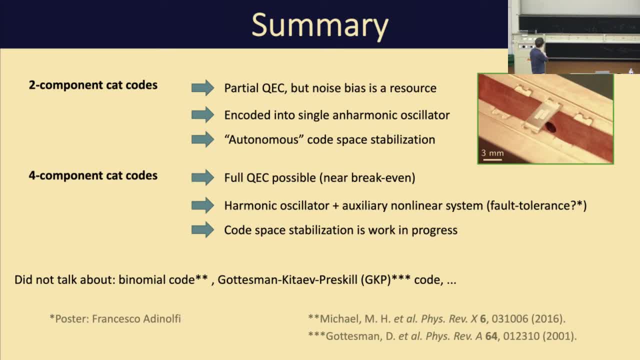 these also stand in with this kind of implementation for a larger class of bosonic quantum error correction codes, such as the binomial code, the Gottesman-Kadaev-Breskell code and so on. There's many more examples in here, for instance: 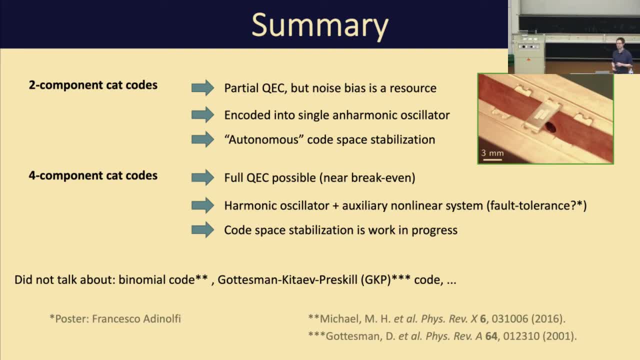 at the summer school you have Victor Albert, who has worked extensively on this, so go talk to him. You have a poster on squeezed cat qubits that have been recently suggested, so there's a lot to learn here as well. With that, I'll just leave up. 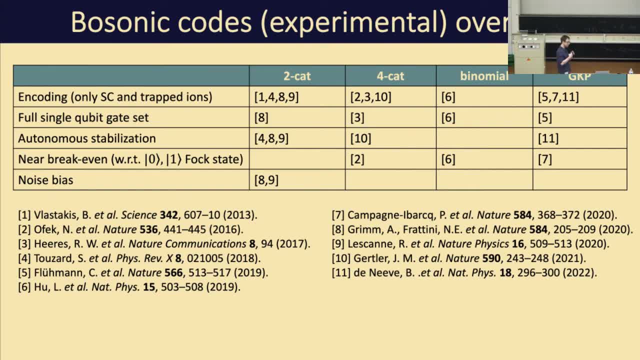 our summer table, where you get a bit of an overview of all the things that have been experimentally achieved, in bosonic codes, for instance. Here I'm focusing mostly, by the way, on superconducting circuits and trap science. that are really the most important. 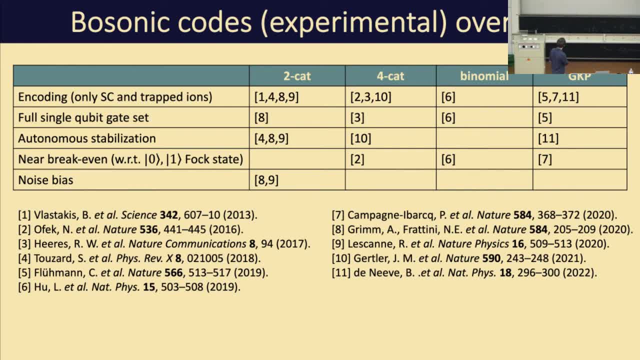 and the leading technologies in that field. where you see, for the 2CAT, 4CAT, binomial and GKB, the encodings have been realized everywhere. Full single qubit sets have been realized everywhere, Autonomous stabilization, mostly in the 2CATs. 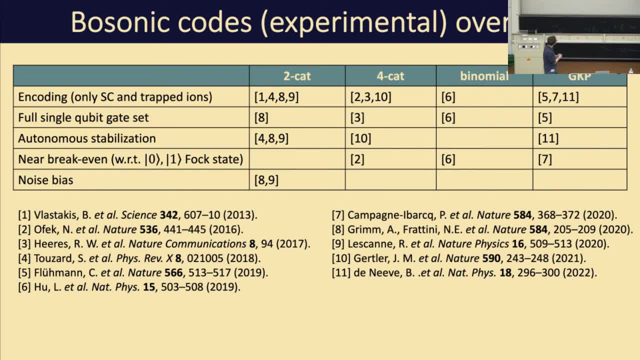 a little bit in the others as well, and then near break even has been achieved for most of these. That's not defined for the 2CAT without having more of them coupled. Noise bias, of course, is the domain of the 2CAT. 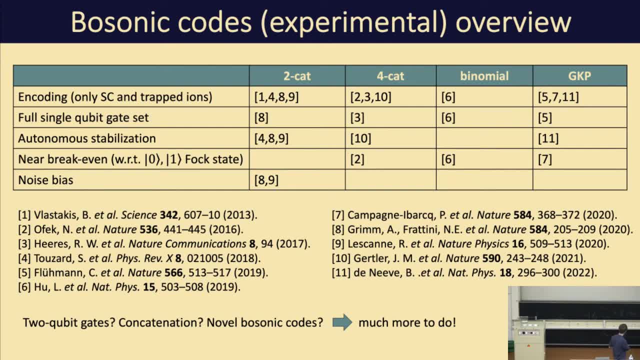 What you'll also notice is there's lots more to be done. I've not talked about 2-qubit gates. I've not talked about experimentally concatenating these Novel bosonic codes. I've only alluded there. There's lots to do. 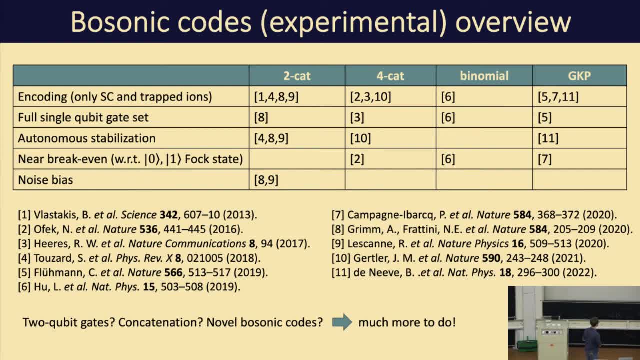 which, in my opinion, is great because we'll actually be able to do interesting experiments that are interesting from a quantum error correction perspective and the physics perspective, because these systems are really nonlinear, out-of-equilibrium oscillators- that are also fundamentally interesting. So with that, 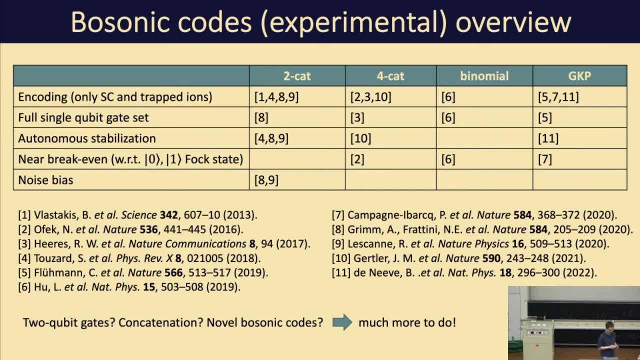 I'd like to thank you, and I would be remiss if I wouldn't mention that we in our new group, which will start in July, always have positions for master's or internship students available, So if you're interested, reach out. 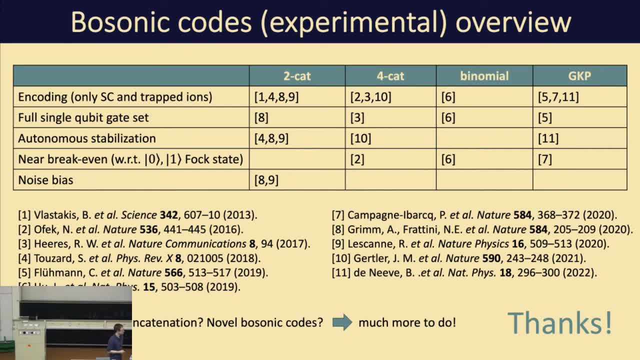 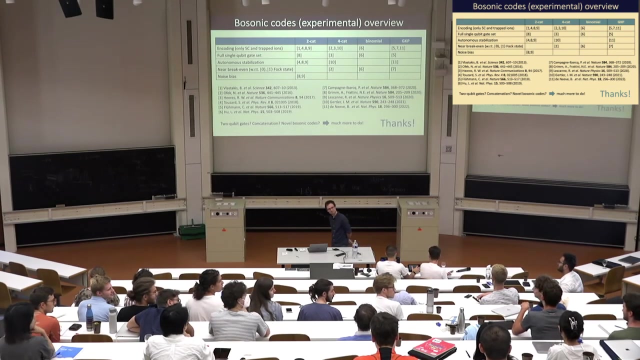 Thanks. Okay, we have time for one question, Thank you. Do you approximately know how you would implement the two-qubit gate? Because actually I would maybe like to do your two students to implement this in the hands-on session. It should be possible. 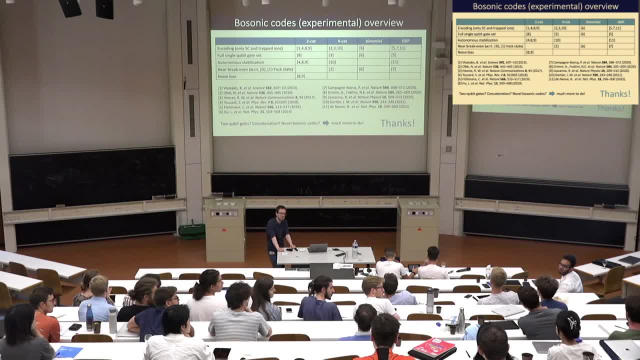 I think if you can write on Hamiltonian properly then they could try this. I don't know if you want to do it, but it would be nice. So I mean essentially for the Kirchhardt qubit I mentioned at the beginning. 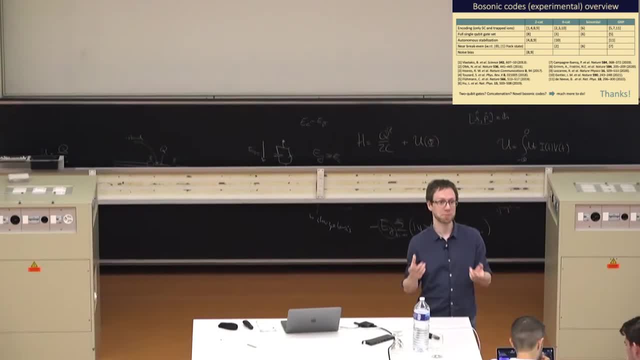 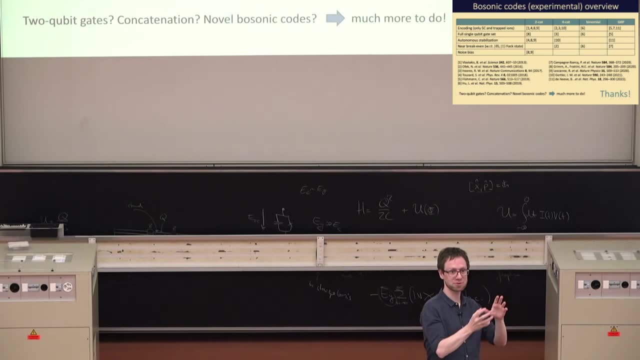 a two-qubit gate. one potential one is implemented by a beam of light, A beam splitter. right, If you have a beam splitter between these two, then if you project that interaction onto the code space of one, it comes down to a sigma z operator. 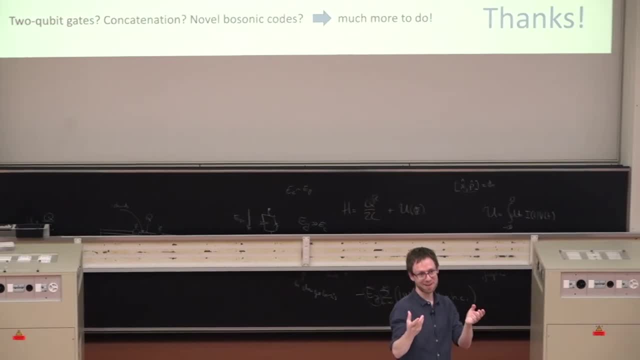 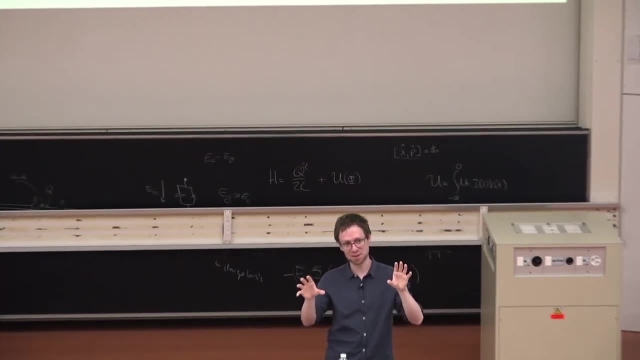 in that and also a sigma z operator in the other, And that will then you know this interaction already- will give you a two-qubit gate. There are also more complex gates that are based on conditional phase-based rotations. Let me see if I have some. 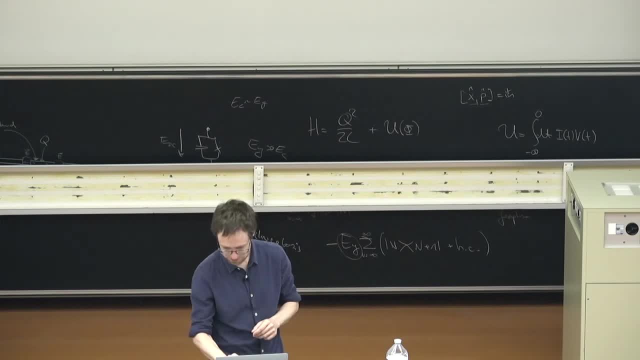 backup slides on this that make this a little bit more concrete, But they are potentially a little bit trickier to implement. They require relatively complex Hamiltonians and parametric drives, So in terms of the physical overhead required for these, you don't need so many parametric drives. 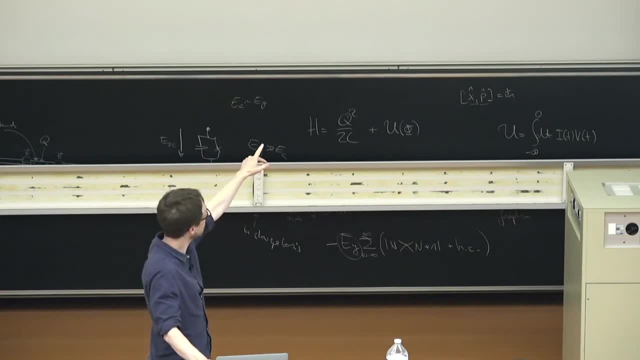 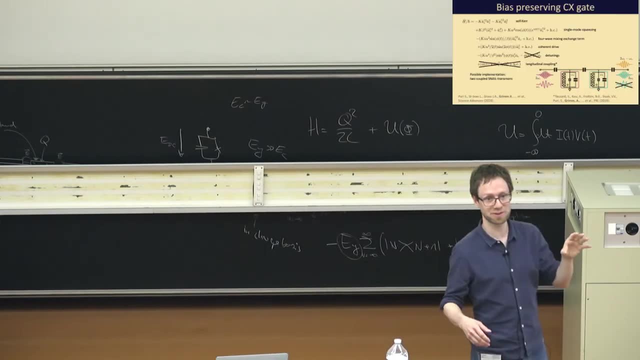 you just need the stabilizations and coherent drives and then another four-wave interaction between them. What's special about these gates is that they are error-biased. preserving which means that you have this noise bias right. Imagine you had a standard qubit. 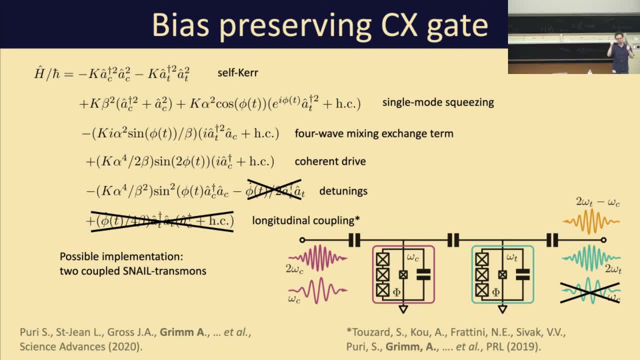 with just two states. that has a noise bias. If you move from one state to the other, you always go through states that are exposed to errors. With cat qubits you don't have to do that. You can just rotate around and phase-base and keep the distance. 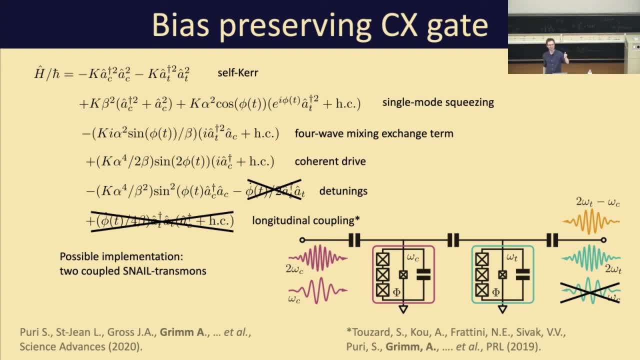 between the coherent states the same, But maybe we should discuss. if you really want to explore an implementation of maybe the simpler gate, we can easily discuss after this. Yeah, Is there somebody? it looks like we do have one or two more minutes if somebody has a question. 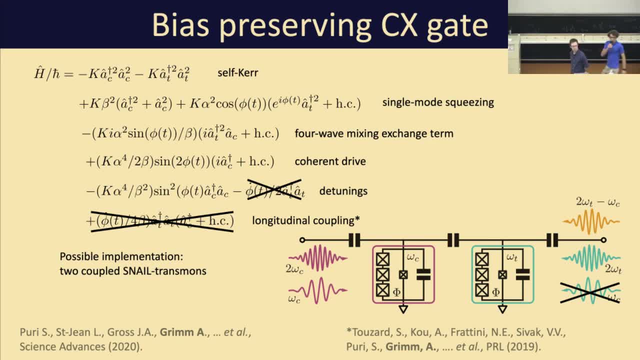 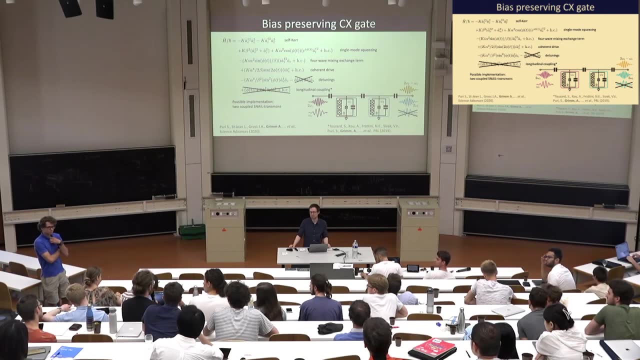 we can take a second And also questions for Cornelius. Yeah, I also have a question concerning these cat qubits. You said that it's possible to detect as a result of this encoding. what would the correction operation be then? Right, so 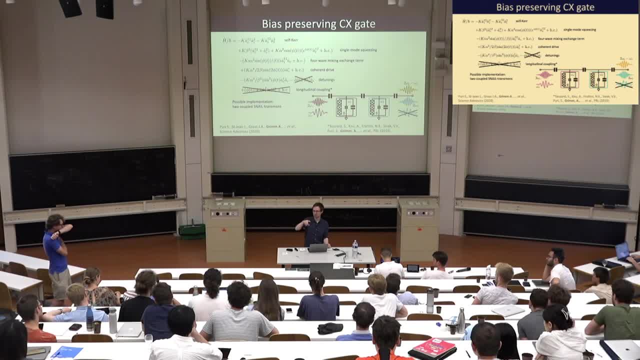 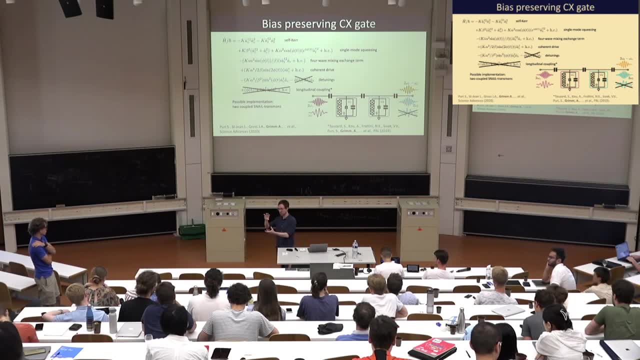 as I said, with this jumping around block spheres, right in principle you don't need to do a recovery operation because you know where your quantum information is Right. It just has changed the basis, Right? But if you then want to decode it, and that's maybe, 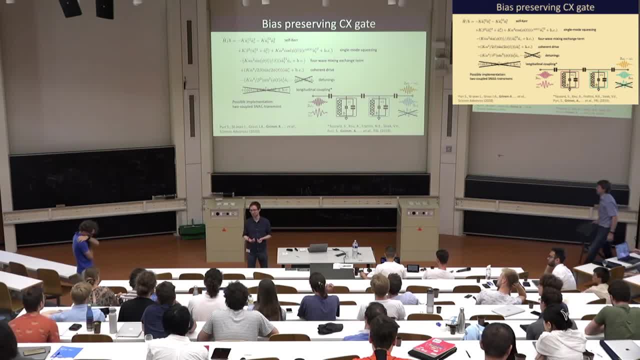 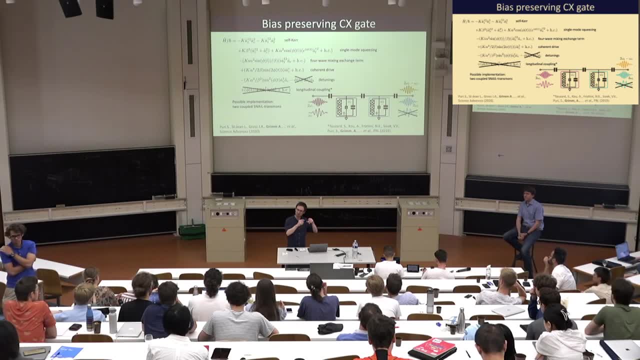 the question that you're asking: how do you decode it? then you have to take that into account, And the way that decoding is done is using again this strong dispersive interaction. you can kind of use a similar protocol, like the one for the parity measurement, where you map. 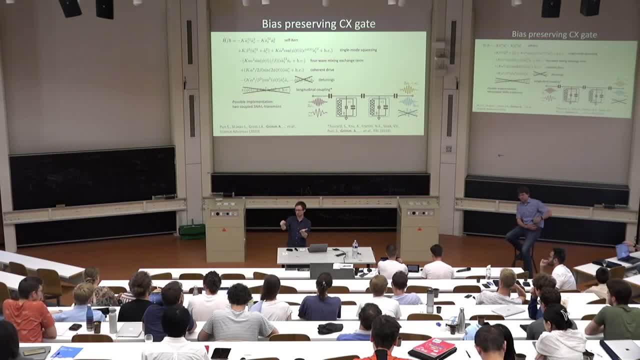 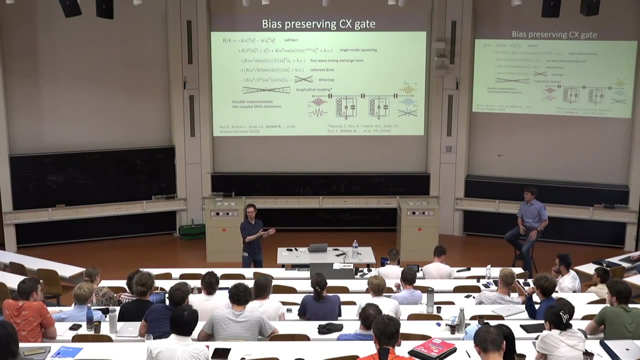 the state of the cat qubit onto the trans one and vice versa. You can maybe feel how this entangling between the two gives you the possibility to do that, And there are actually more sophisticated protocols now that have been, you know, essentially adapted from NMR. 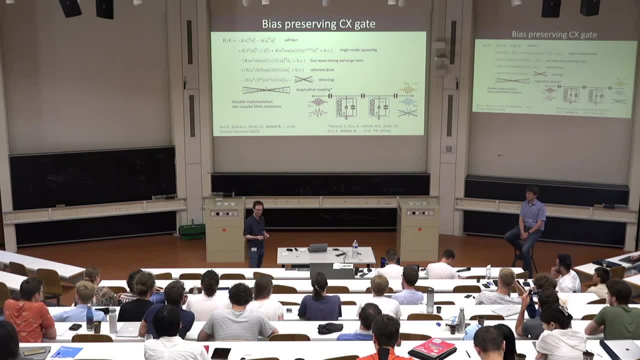 Cornelius has mentioned this earlier. We have heavily drawn on the field of NMR, where you can do optimized controls or really optimized both sequences that perform decoding operations in a way that on these kind of bosonic qubits, and it's actually quite impressive. so this is an example. 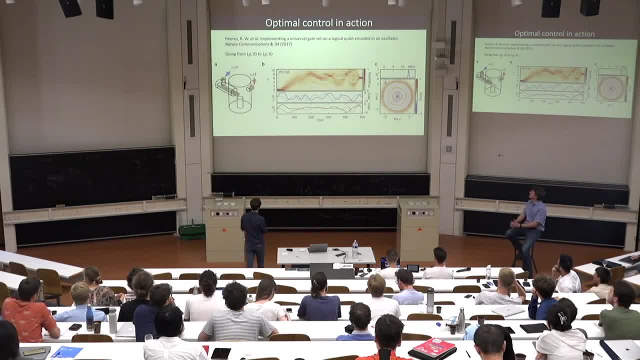 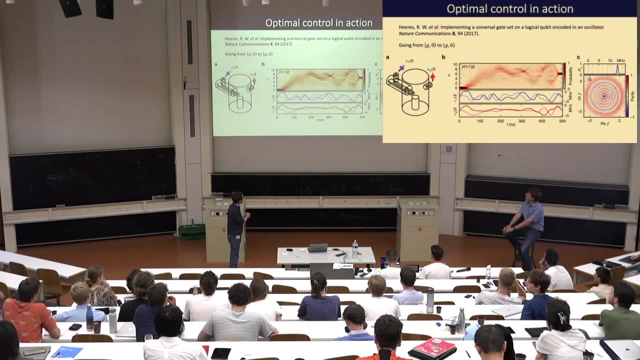 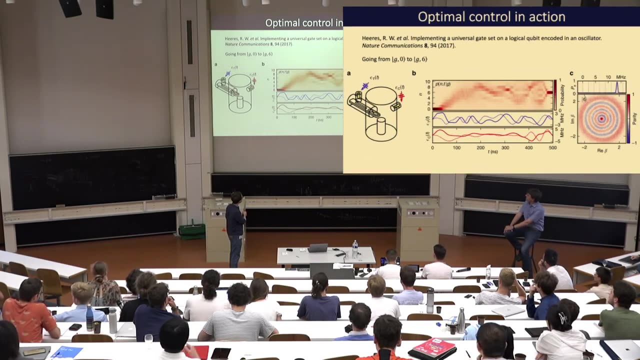 of such a such a pulse sequence. It's really numerically optimized. You're applying drives on the auxiliary trans one and on the cavity with some completely great shape, and this is what happens to your cavity during this. so it starts in the ground state, in the zero state. 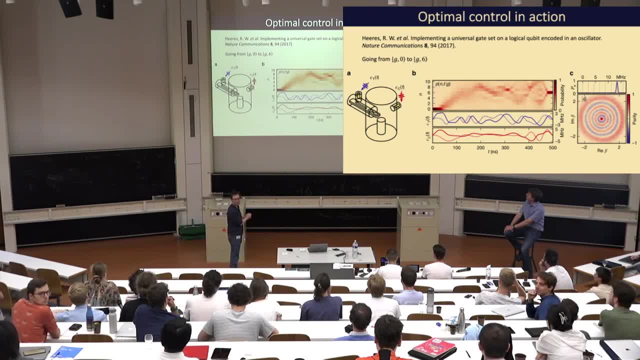 and then it goes to some crazy states and then it ends up boom in the six photon state. so that's an example of how you make a six photon state with these kind of then there are again questions in terms of fault tolerance and so on. so it's still. 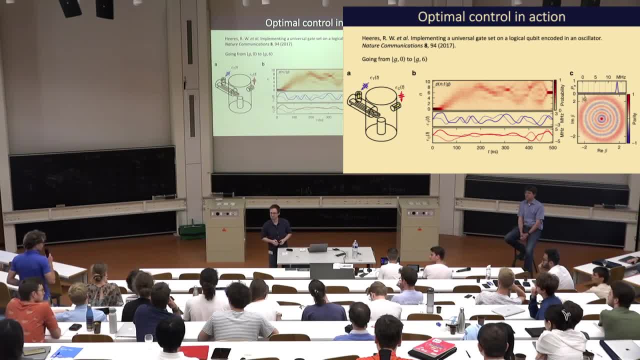 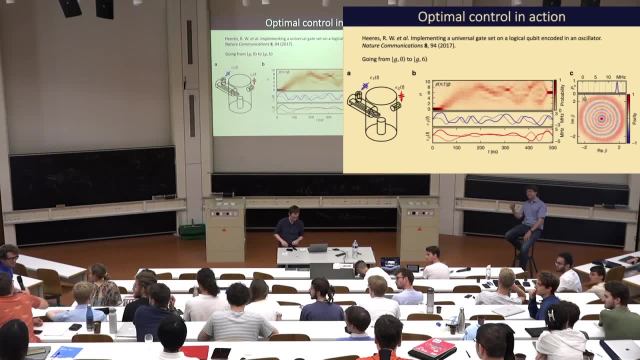 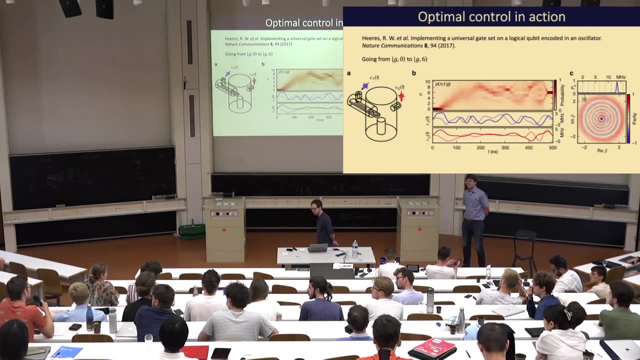 as I said, an active field. One question for Cornelius: Hi, So you've talked about the scalability in terms of the hardware. I was wondering whether you could comment. so, if we look, for example, at your 2018 PRX paper on the scalability, 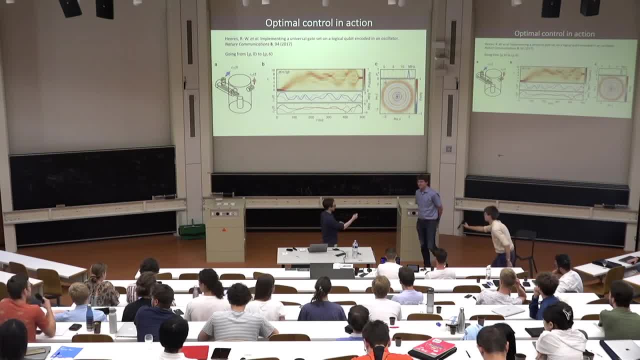 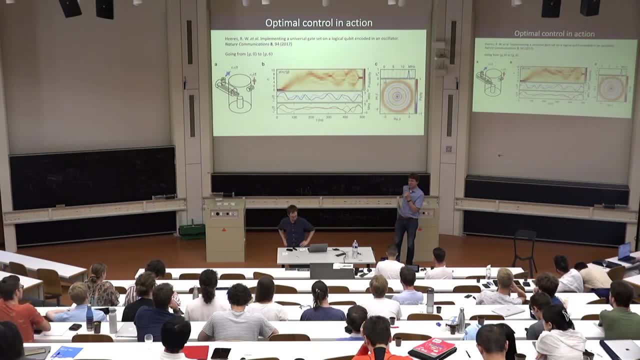 of those applications and how, in the way that they were implemented in that paper. so let's say, the generic VQE for chemistry. what's your opinions on the scalability of that? I sure can. Yeah, so the 2018 PRX. that was this quantum chemistry. 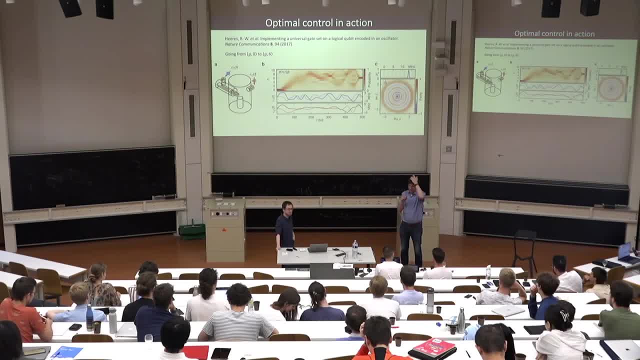 variation of quantum eigensolver paper that we worked out and I think you know I should give you the truth on quantum chemistry and VQE, and that is: do not expect a miracle anytime soon unless there's quantum error correction. hence also my shift to really scale this up. 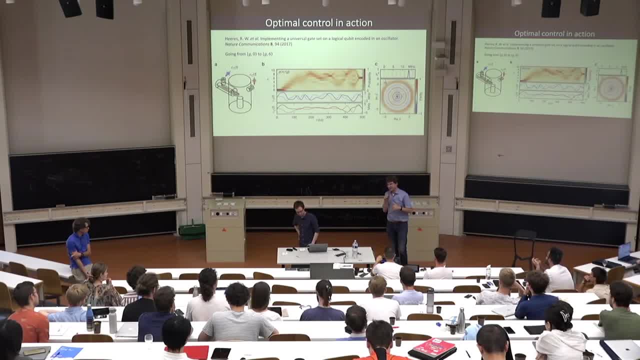 and if you don't believe my words, you can find there's, I think. the Simons Foundation hosts talks at Berkeley, and Ryan Babish, who's the head of algorithms at Google- this close colleague- we worked this out in 2014 and really went through it. 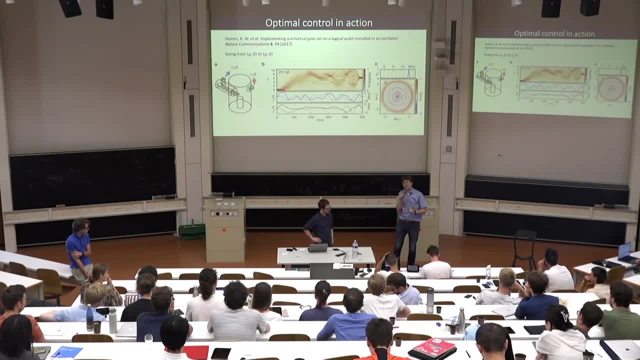 Google implemented it, IBM had their nature cover and all that, and even Ryan, who's the most optimistic person in this space. like he we talked. you can do two qubit gates. that's your fidelity. awesome, we can do water. let's do water straight away. INQ has tried. 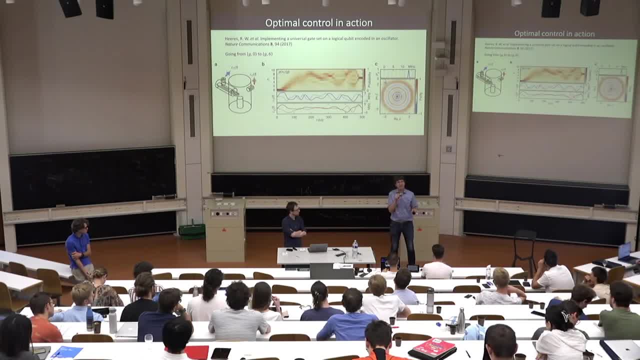 water. they've done a little bit of it, but not really there and by far not at the accuracy level that you need, and I think there's not sad truth, but the way why chemistry is a very good benchmark is because chemists are pretty good at calculating things. 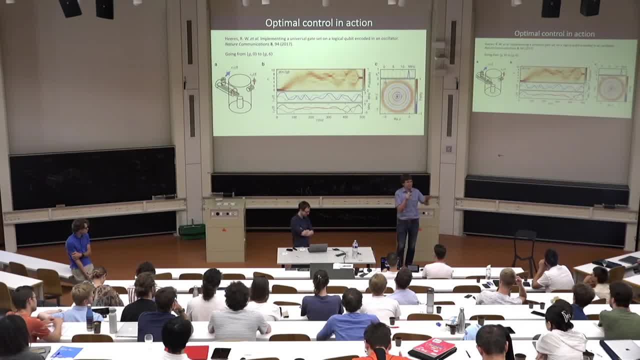 they've had 50 years of quantum chemistry and really good calculations and approximations. so when you think about hydrogen, which was one of the things that we did in this paper, you know, you write it down, you know this even in your undergraduate classes. you know quantum mechanics. 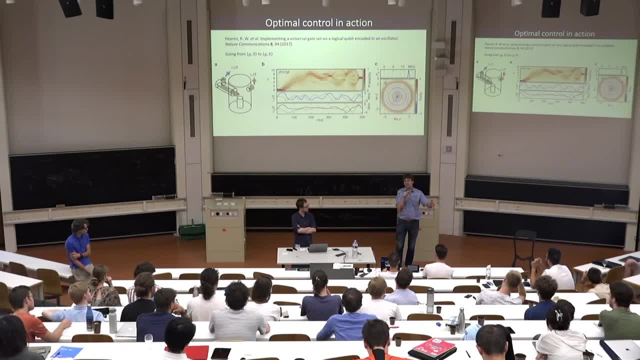 hydrogen. you can solve it. you can go to your 12th decimal digit and I think he once talked to a chemist and he said: oh, 18th decimal digit, not a problem, your quantum computer has 10 to the minus 3 error rates. how do you think? 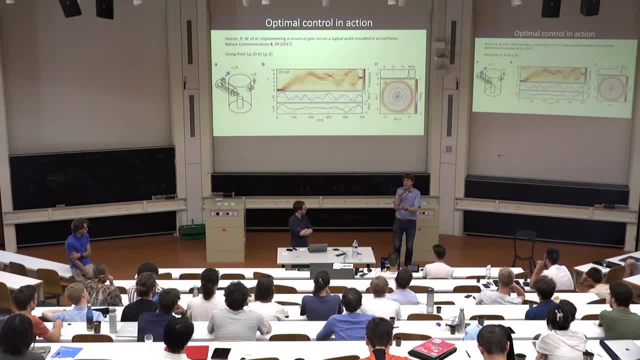 you're thinking to 10, to the minus 12. so even Google now admits 20 qubits is likely going to be the limit, and they had a recent paper- I think it was in science even- on using again an approach like this to simulate a larger hydrogen chain. 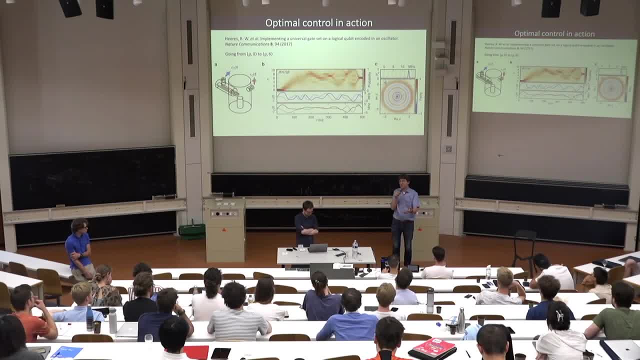 and also carbon and also there, you know, the bottom line is it's not good enough. they need to do post selection and once they get to 12 qubits on the Sycamore chip, that's it. you know, you're no longer chemically accurate. 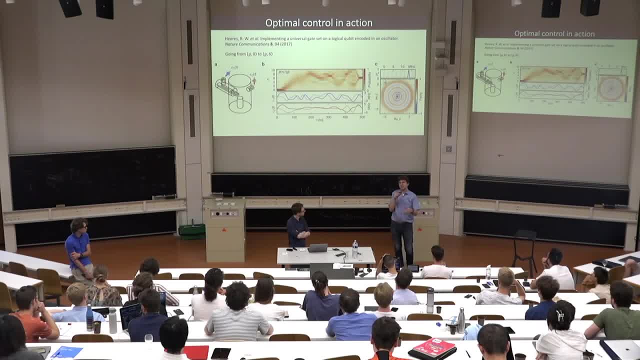 and any chemist will turn your back on you and immediately leave because you're no longer competitive. so you need quantum error correction to get there. but to end up on the positive note, this is what my team in Australia is still doing: analog quantum chemistry, you know. 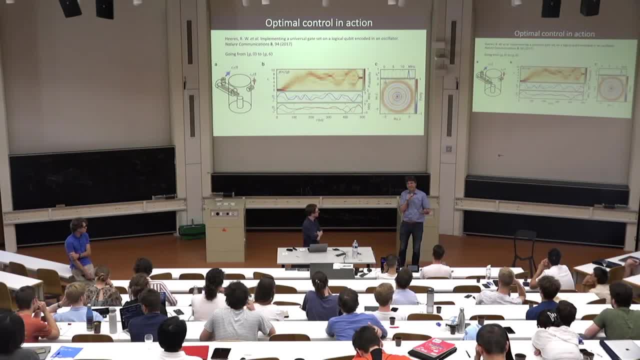 we have an analog device and if you think back to analog computing these days, you know of course it was all about military applications that we probably shouldn't talk about in the current circumstances, but that's really what analog computers were used for: guidance systems you can think about. 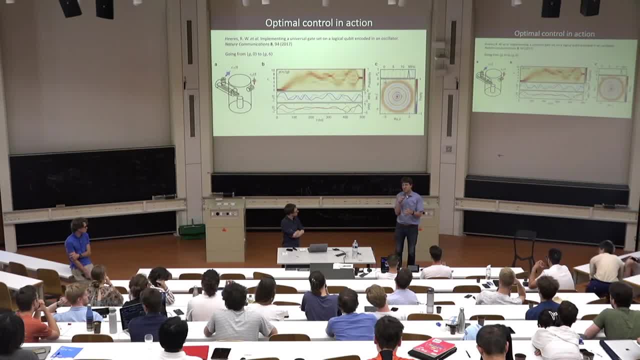 chemical reactions, which is really where the interesting stuff happens. we can solve the static problem. that's what VQ does. static problem, Born-Oppenheimer approximations: only electrons allowed to move around nuclear have to freeze. but that's not where the interesting stuff is. the interesting stuff 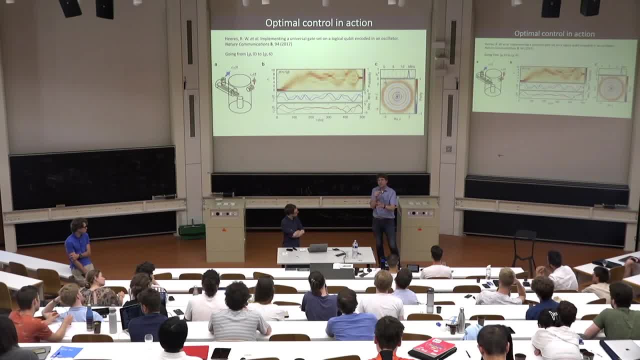 is when the nuclear move. now you have a quantum system where there are vibrational degrees of freedom and trapped ions. that's why we love doing this, also in Sydney. currently you can use those vibrational degrees of freedom, similar to what you were studying, for quantum air correction. 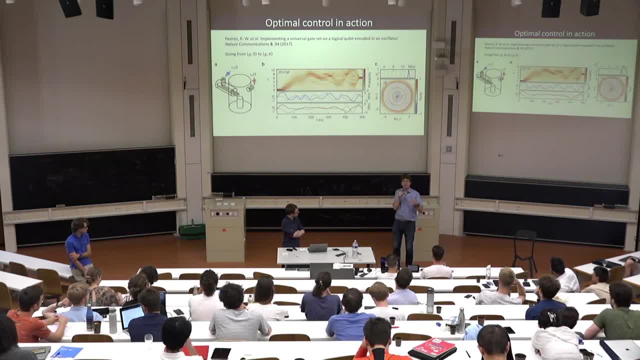 you can just use these. then you're no longer talking about qubits and error rates, you're talking about oscillated degrees of freedom. and then you're talking about an analog simulator, and my hope is that there you can really achieve something- not quantitative, I'm not going to. 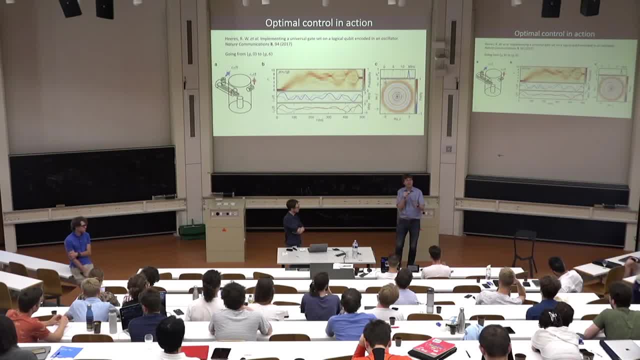 bet down to the something decimal digit, but qualitative. when does a phase transition occur? when does this and that happen and how does this molecule form? so currently we're looking at a molecule, pyrazine, that is similar to retinol in your eye. it's a mechanical switch.